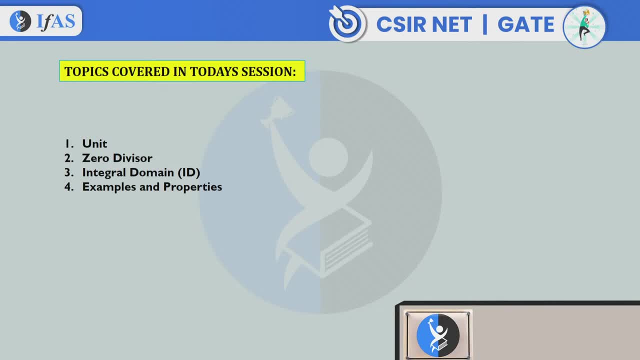 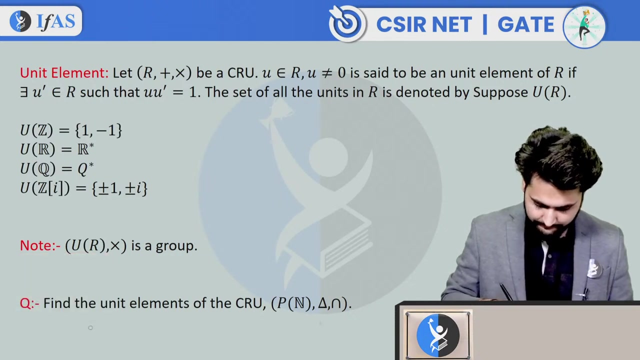 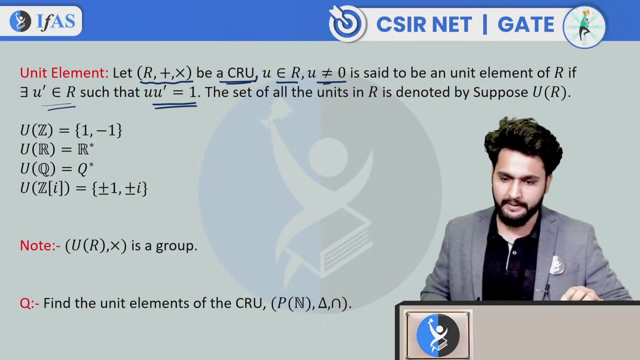 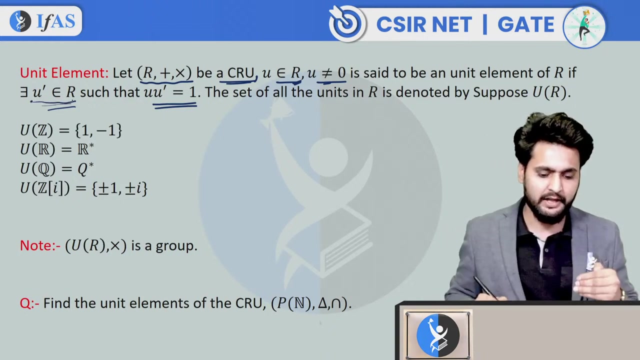 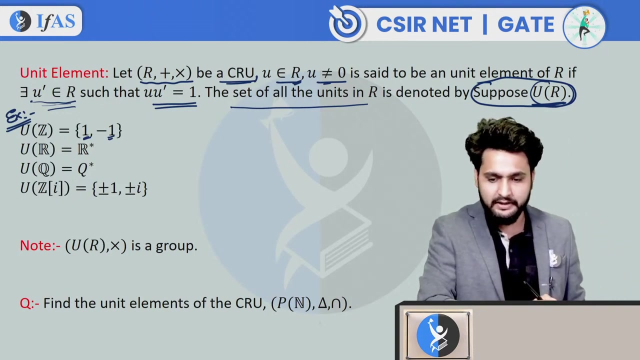 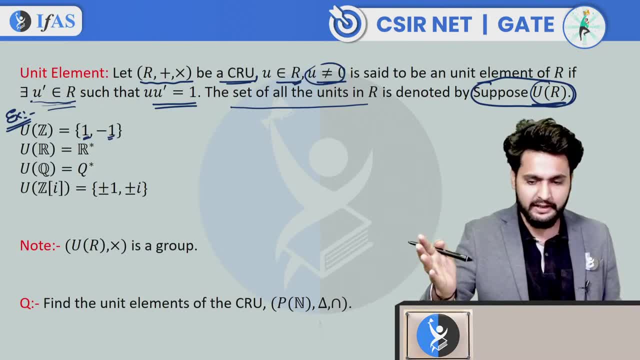 You can multiply anything in zero, but it will never give you 1.. Zero can't happen anyway. Any non-zero element will be called a unit element if its inverse exists. So what are the integers whose multiplicative inverse exists? 1 and minus 1, nothing else. 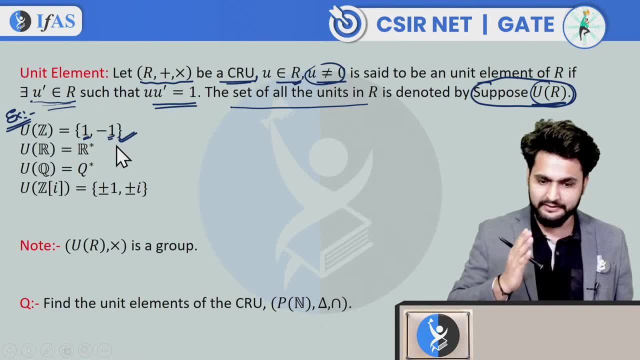 So this is the units of Z. We have noted this in the form of a set. Similarly, if we talk about units of R, R is your field. If you take any non-zero real number, what will it be? Multiplicative inverse. If I take R, let's say R0 equals to 0.. 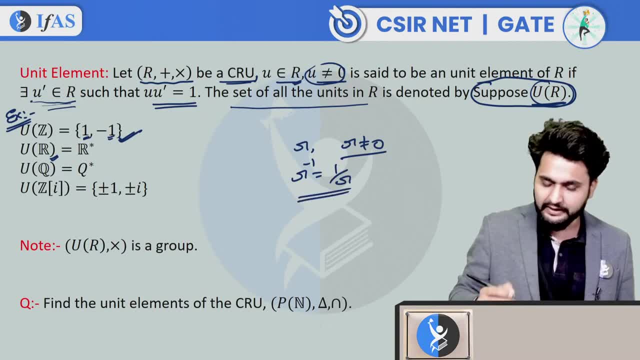 So what will be R? inverse 1 upon R? we can define. This will also be a real number. So how is every non-zero real number? It is your unit element. So R star will be gamma. All the unit elements of R is nothing but. 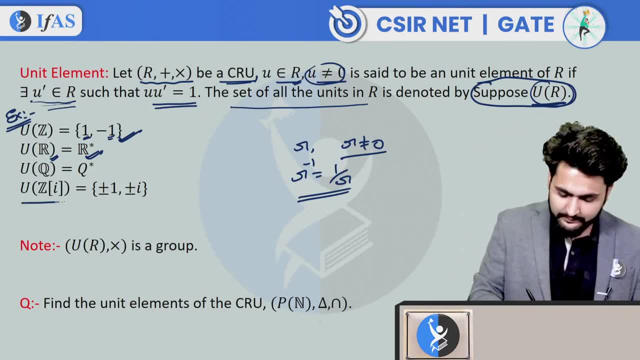 all the non-zero real numbers. Is that clear? Then if I ask you: what are the units in ZI, What are the elements in ZI whose multiplicative inverse exists? So how do we define ZI, a plus ib, where a comma b belongs to Z? 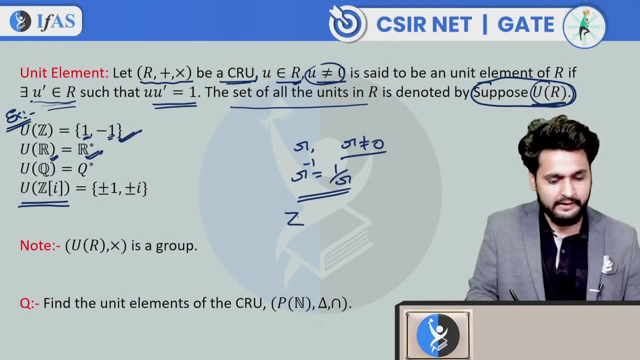 So in ZI there are only 1, minus 1, i and minus i. These are the unit elements. Apart from this, there are no other unit elements. Keep this in mind. Sometimes you will also see such questions: What are the units in ZI? 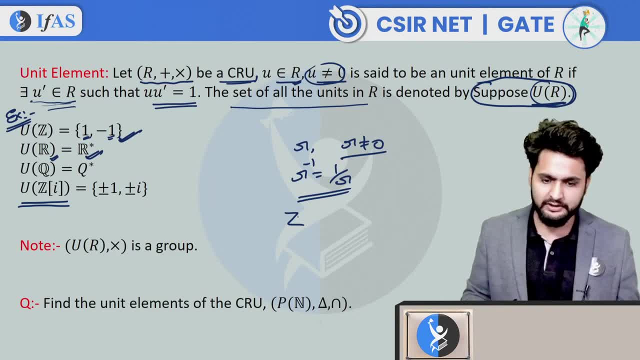 1, minus 1, i and minus i. Their inverse exists, No one else's. The inverse of i is minus i. If you see the inverse of i, then it is minus i. If you do the inverse of minus i, then it will be i. 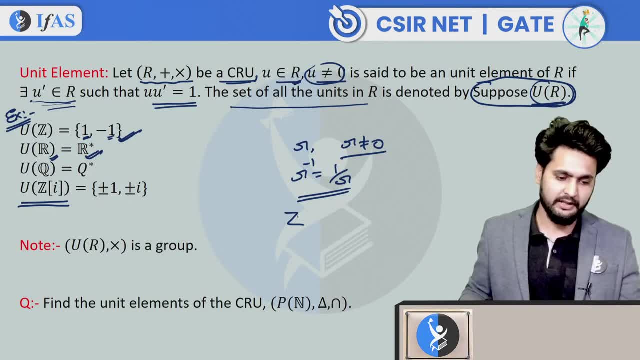 And what is the inverse of 1?? The inverse of 1 is itself 1.. What is the inverse of minus 1? The inverse of minus 1 is itself minus 1.. So we can see that everyone's inverse exists. And these are the only unit elements in ZI. 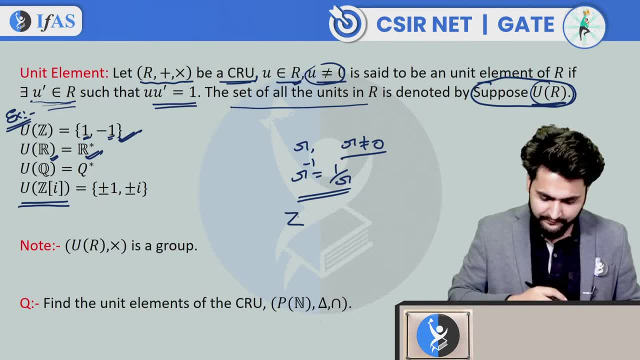 Is that okay? So these were some examples for unit elements. Let's move ahead. You can see that UR, with the operation multiplication, is a group Group of unit elements. in any ring with respect to multiplication will become a group And there is nothing new in this. 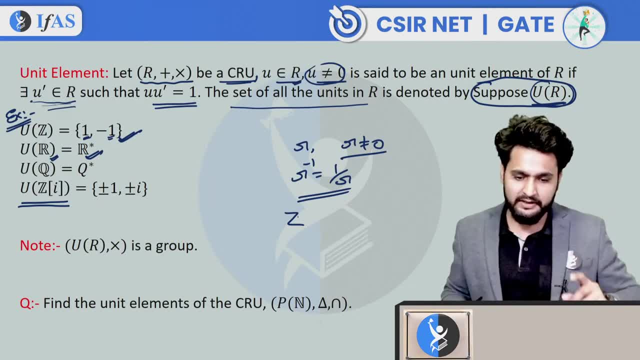 If you know the definition of a ring, if you know the definition of a group, then you can easily verify this. Good evening Ajit, Good evening everyone. Fine Units, this is a group. What all do you have to verify in this? 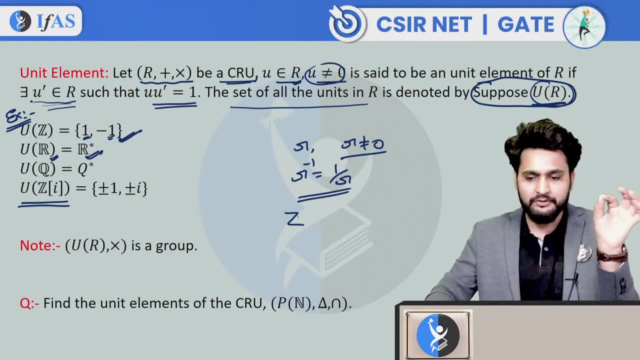 See what happens. for a group. The first condition is closure property. So if there are two unit elements, let's say U, and I have taken U1 and U2.. These are two units, Their inverse exists. So the inverse of U1 and U2 will also exist. 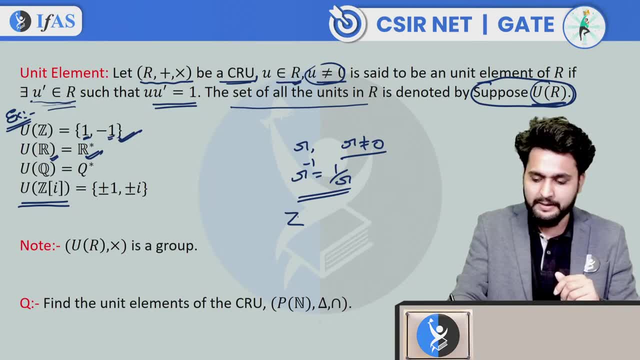 What will happen to it? U2 inverse into U1 inverse. What is the problem? Closure property is done. Good evening Shatna, Good evening everyone. Is that okay? So closure property is done If there are two unit elements. 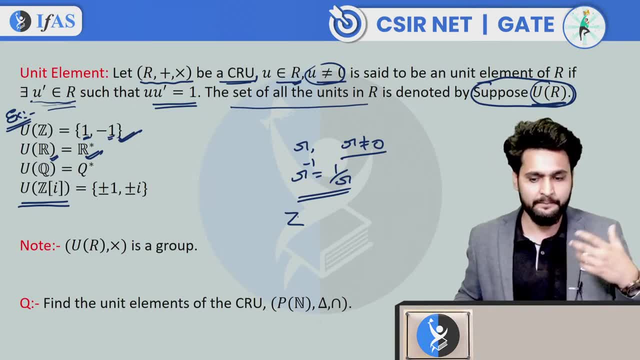 then their multiplication will also be a unit element. We will get a unit element even if we do their operation. Then what is the property after that? After closure property, there is an associative property. So multiplication and associative are in the whole ring. 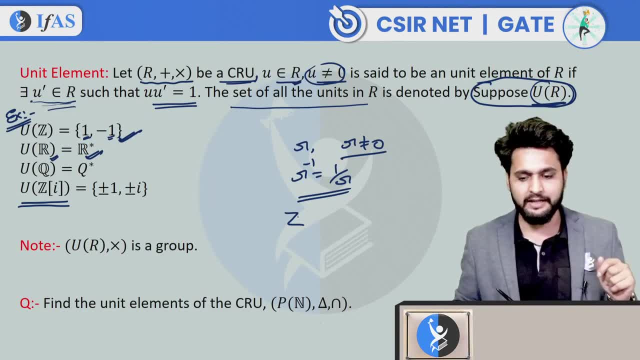 So this will also come in it. This is its subset. So multiplication and associative is done. Then what do we have to do? Existence of identity element. If 1 is near the ring- and that will happen- then we will define the unit. 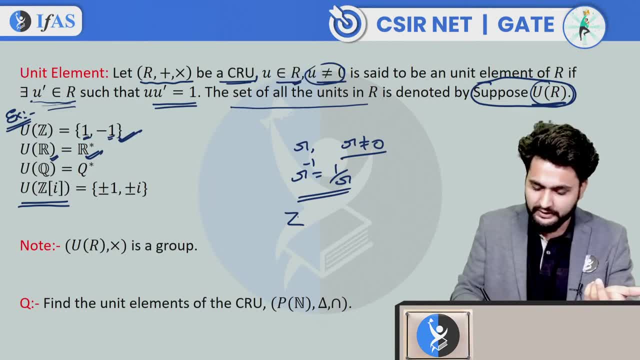 So 1 always has an inverse, So 1 is always a unit element. What will be the inverse of 1?? 1 will be itself So unit element. unity, identity will also always be in it. Then what is left? Inverse element? 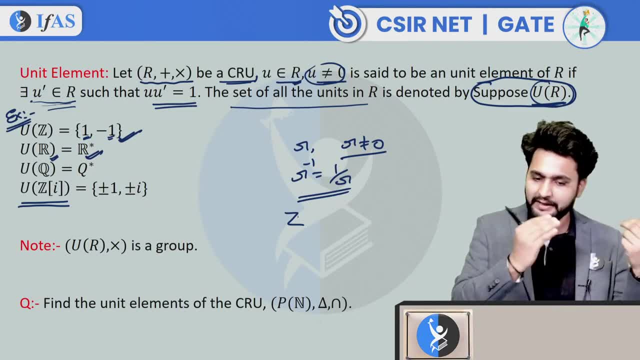 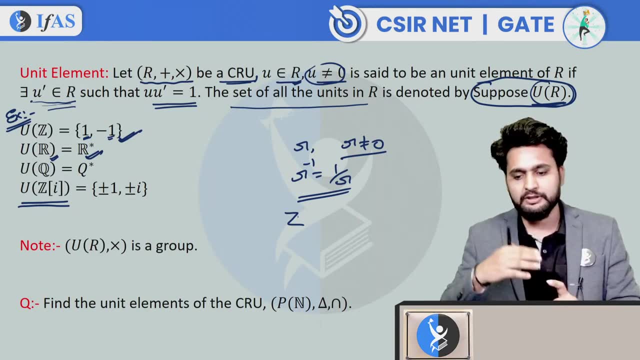 We are taking the property of inverse Right. We are taking the same element whose inverse will exist, So that will also be in it. So a group is made or not. So if the collection of units is done, then in respect of the second operation, 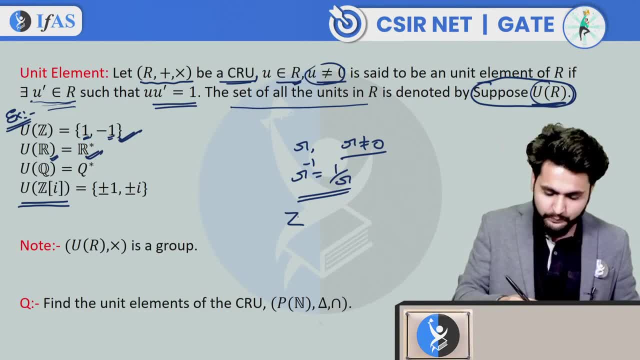 a group is made. For example, you can see whatever is written above. are these groups or not? See, You have taken units of z. Is this a group or not? There are two elements in it. Is this a group or not? 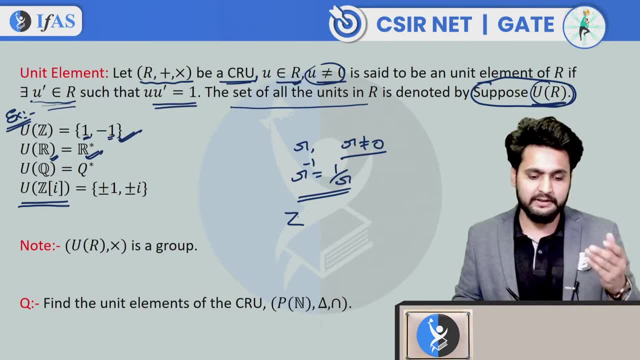 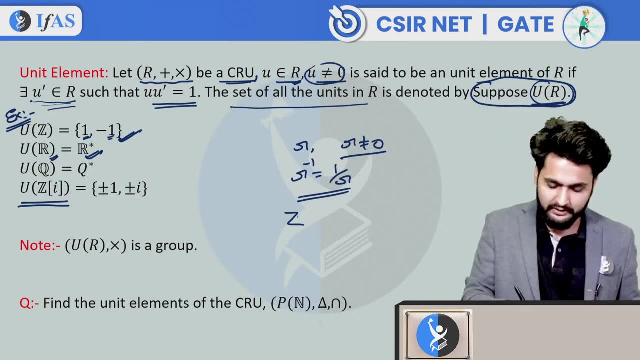 Absolutely it is a group. If you see this r star with operation multiplication. is this a group or not? Absolutely it is a group. Good evening everyone, Fine r star with operation multiplication. is this a group or not? Absolutely it is a group. 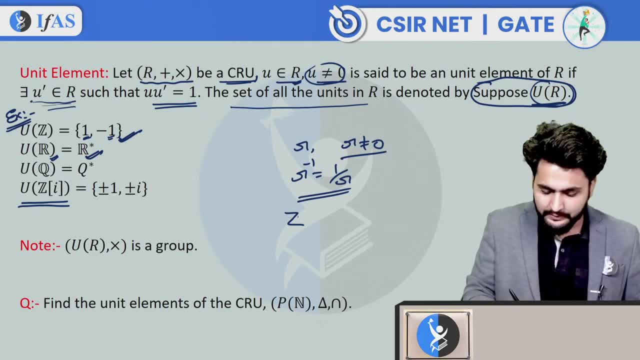 q star with operation multiplication. is this a group or not? This is also a group. Plus minus 1 comma. plus minus 1 minus i. This is nothing but the fourth roots of unity. Is this also a group or not? This is also a group. 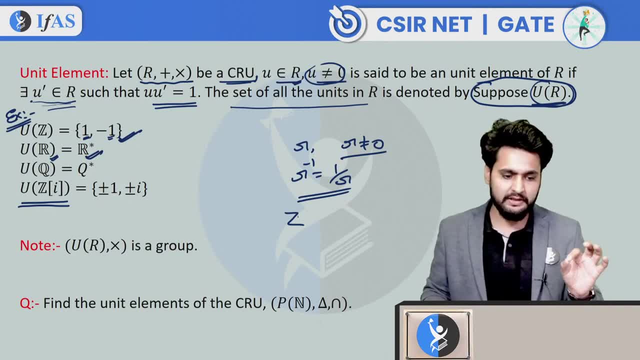 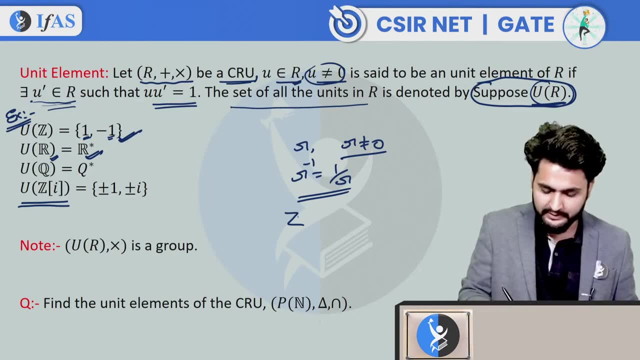 So are all these groups made or not? So you have to keep this point in mind. Units of any ring are always forms a group with the second operation. The second operation may be changed too. Here they have written multiplication. Multiplication is just a notation. 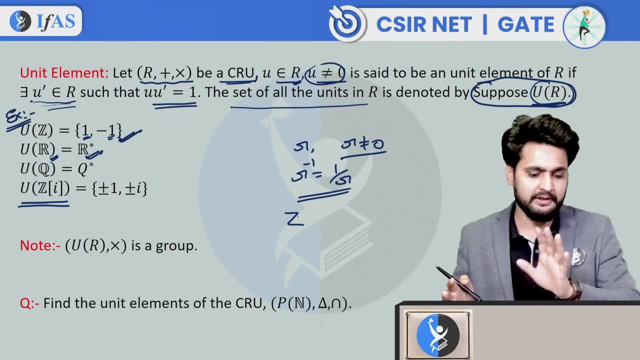 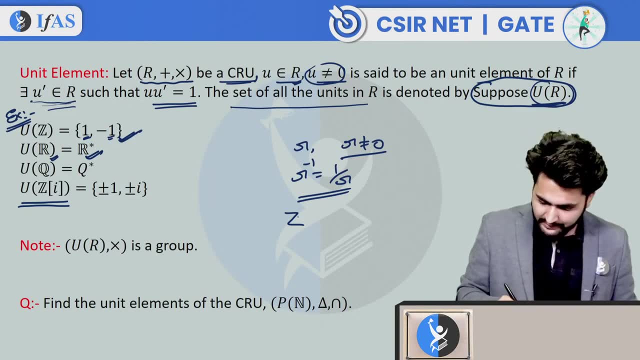 Whatever second operation will remain in the ring. in respect of that operation, the collection of units becomes a group. Come on, See this question and tell me the answer of it. Find the units of r star with operation. multiplication. r star with operation. 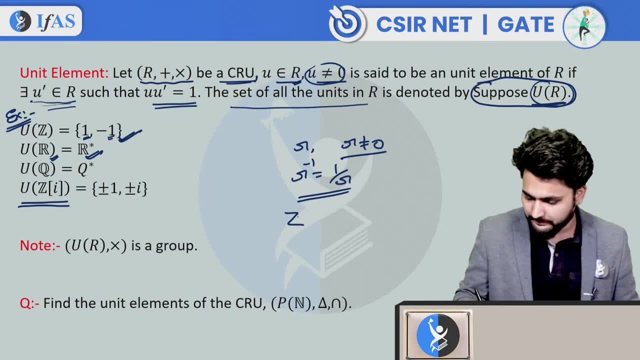 multiplication unica, elements in the CRU commutative ring with unity, power set of natural numbers with symmetric difference and intersection operation. What is the power set? Give me a second. I will add one page. What is in power set of natural numbers. 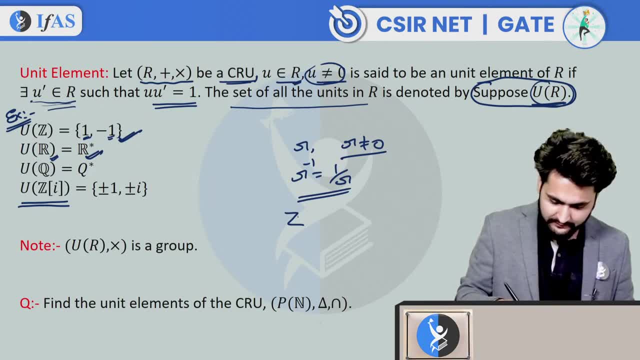 Subsets of natural numbers. So which subsets of natural numbers are there? whose inverse will exist. Can you answer this? I will add one page. Give me one second. Tell me Right. How is power set of n defined? What will happen in power set of n? Let's say, a belongs to power set of natural number. 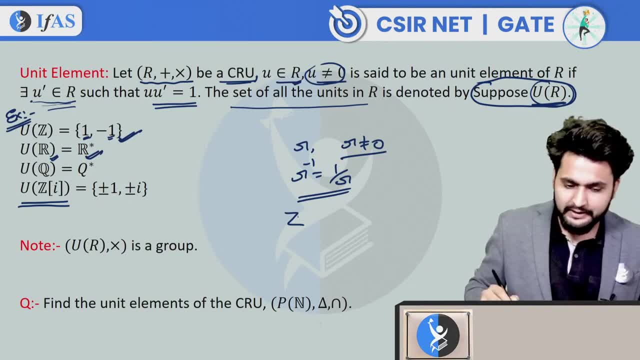 What does a mean? a is a subset of natural number. Now, if we want to see its inverse, whether it is a unit or not, then we have to see n, only. So now we will see that. So what we have to see is: with whom does a have an intersection? 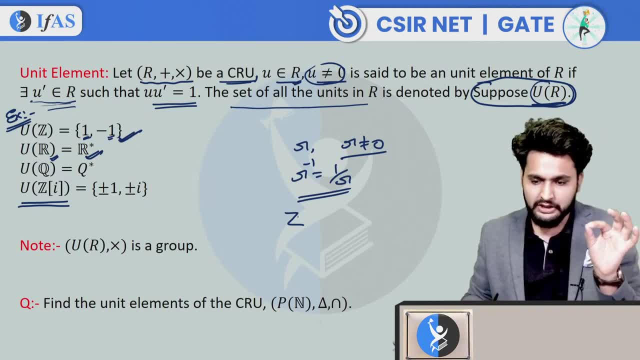 Means: will any such element exist? Element means: will any such subset of natural number exist, So that when we take an intersection with a, it becomes an identity element? First of all, we have to see unity. what is its unity element? 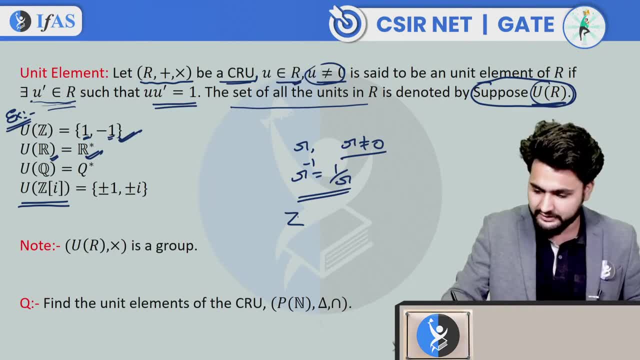 And the unity element. perhaps I have already told you that n itself, n is a subset of n, So this is also a member of power set of n and belongs to power set of n. Right, If we take its intersection with someone- a intersection n is always equal to a. 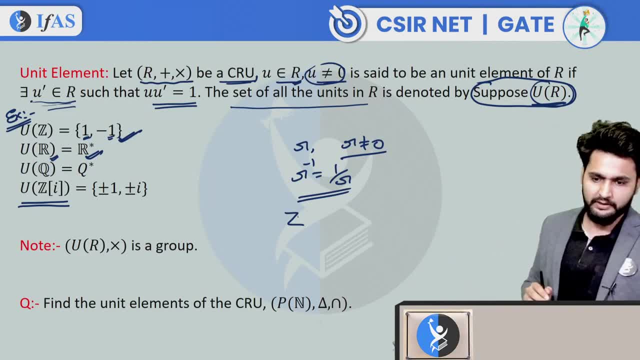 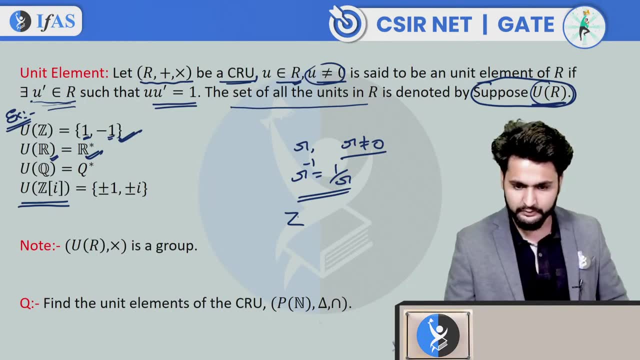 Means we have to take an operation with someone, But there is a second operation. Why can't you see this One second? what is this? Just a minute? Perhaps you can't see the screen? Give me one second. Give me a minute. 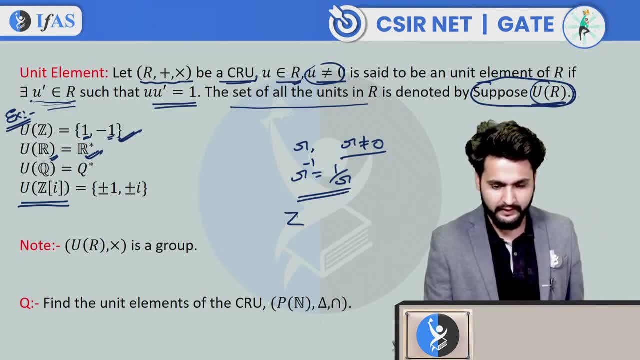 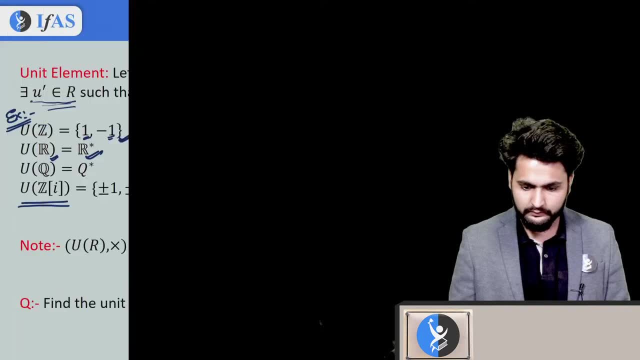 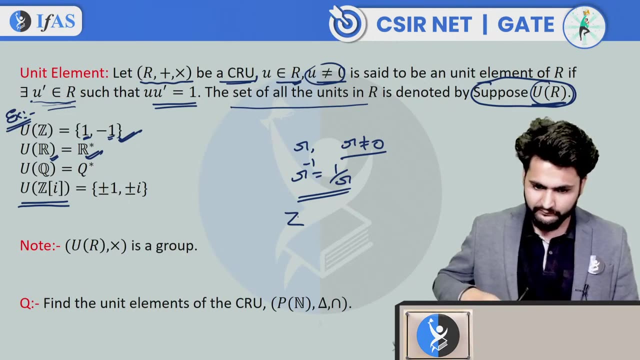 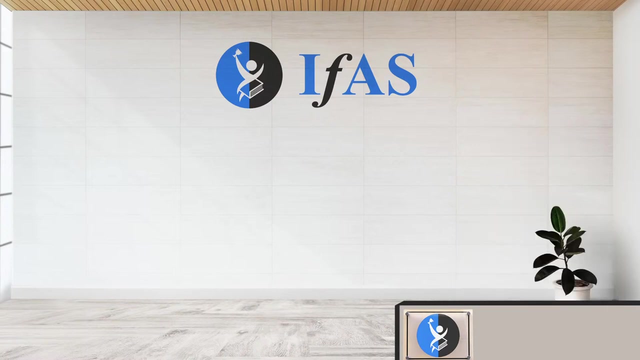 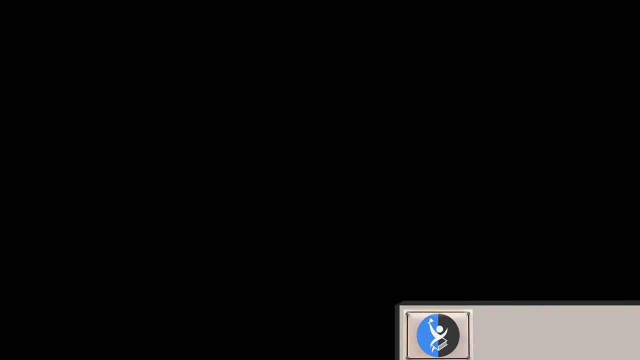 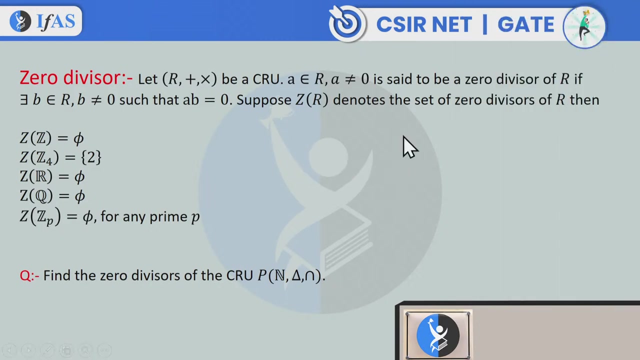 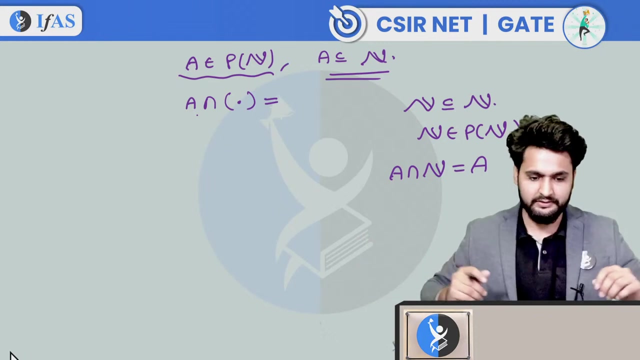 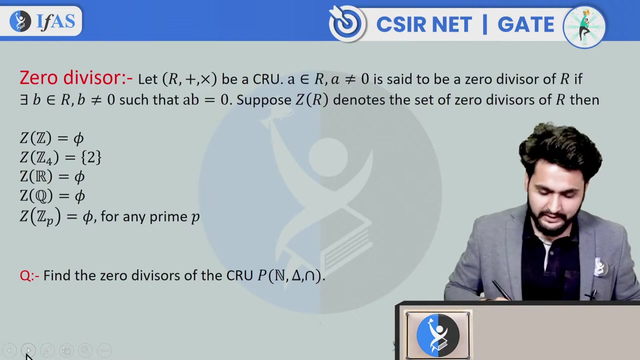 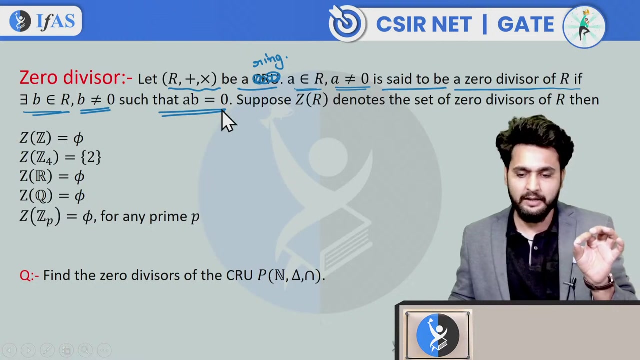 Only n. there will be no one except n. Okay, fine, we will see. that means it is zero divisor any two elements which are non-zero. if they are zero, it means both are zero divisor. 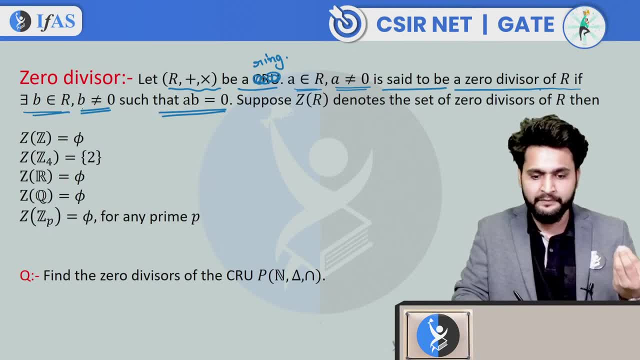 a is also zero divisor and b is also zero divisor. ok, so those elements which are non-zero, and if they are zero in product, then we will call them zero divisor. suppose Zr denotes the set of zero divisors of R, then Zr I am just denoting. 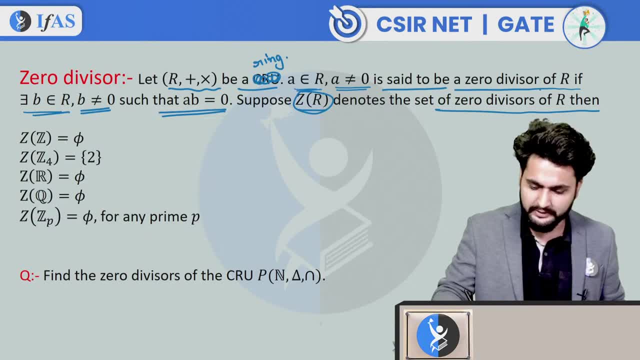 that if the collection of all zero divisors of a ring is done, then let's say Zr is denoted, for example, in integers. if you see how many zero divisors are there in Z, which elements are there which are non-zero? and if they are produced then they will be zero. 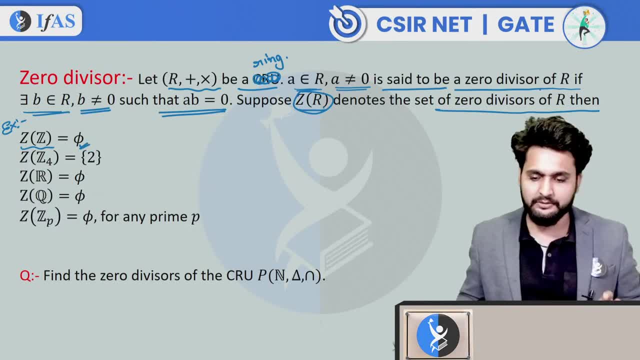 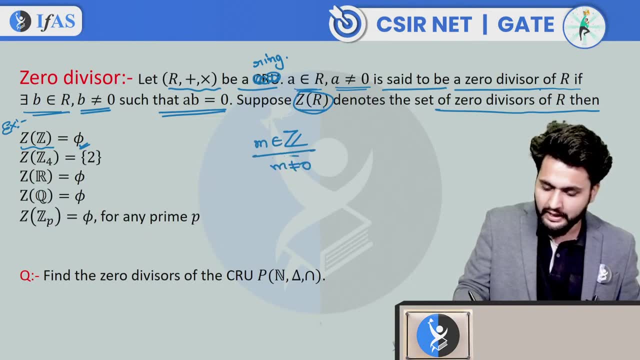 so Z of Z. if I take out zero divisors of Z, then what will come? pi will come. nothing happens. it is in Z. if you take any, let's say m belongs to Z. m is not equal to zero. so if you produce any, 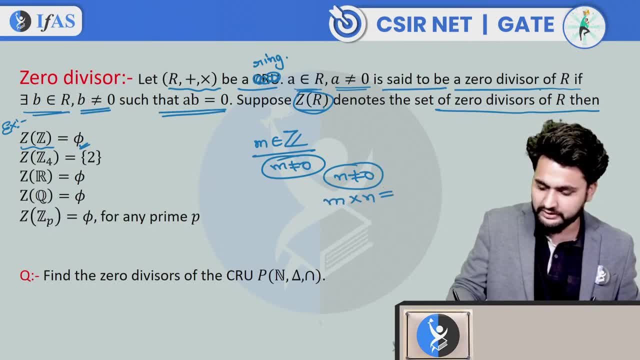 n not equal to zero, m into n will be zero at any time. this is not equal to zero. m into n is equal to zero in Z. if, and only if, m is equal to zero and n is equal to zero, then this is not possible. this means how many zero divisors are there in Z? 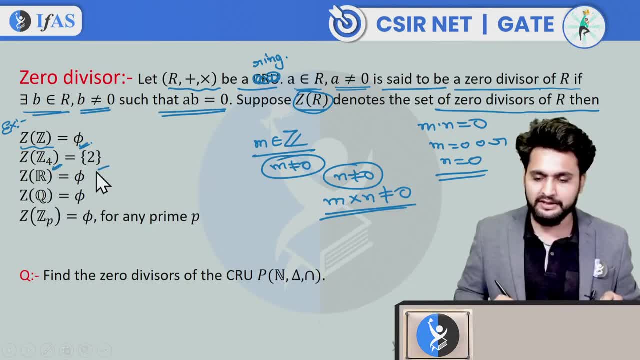 five, right after that in Z4. if I ask you, how many zero divisors are there? what elements are there in Z4? Z4 has zero comma, one, comma, two, comma, three. these elements are there. so if you notice in this the elements units, you know. 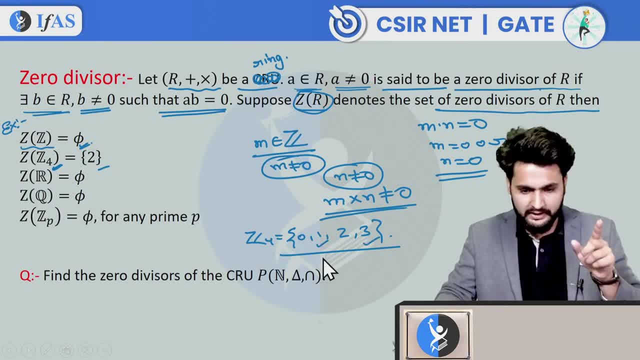 units of Zn like you make un group, so one and three are unit elements. we are going to discuss this now that in Zn or in general in any ring, if there is any unit element, then it cannot be zero divisor. if there is any unit element, then it cannot be unit element. 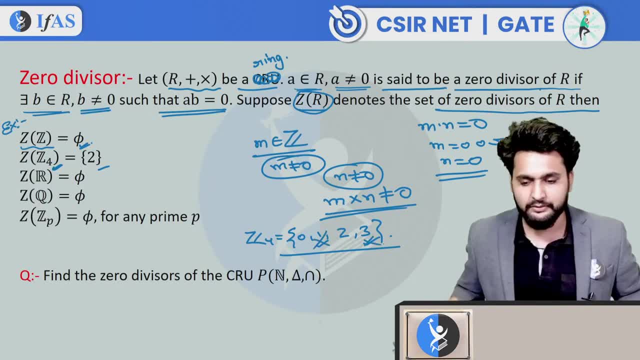 so this is a unit element. so this cannot be zero divisor. zero divisor never happens. what is left is two. let's check two. so if you do two into two, then you will get four. so two is a non-zero element. if product is zero, then it means it is zero divisor. 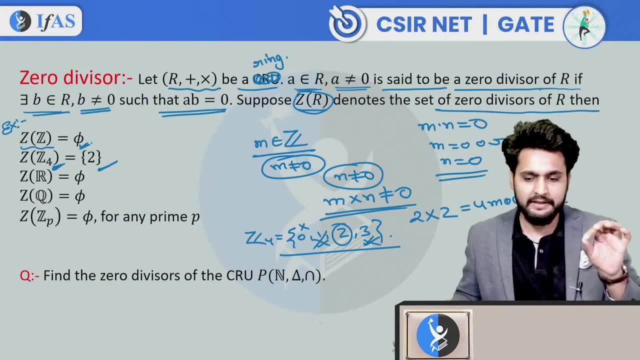 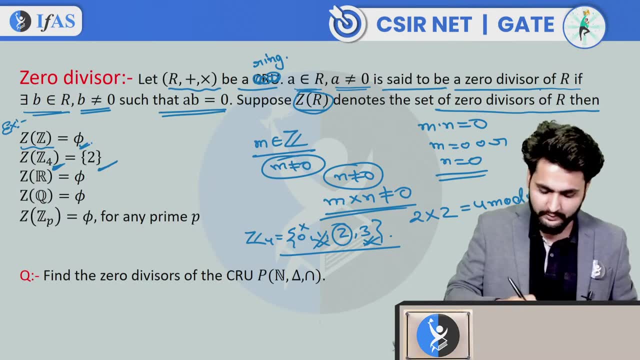 so how many zero divisors are there in Zn? two zero divisors are there, so you can get all zero divisors. you can get zero divisors. you can get number of zero divisor. we will discuss this later. if I talk about set of real number, 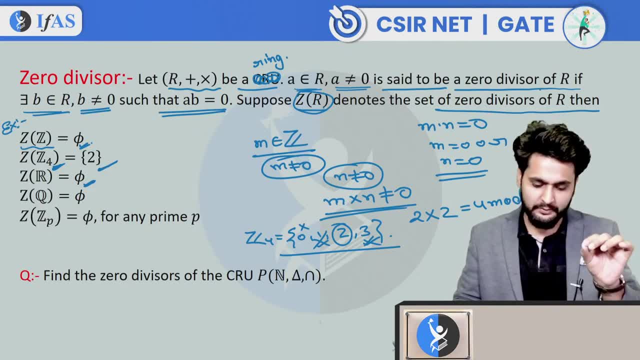 real number is a field and there is no non-zero element. like I told you, there is no unit element. if I talk about set of rational number, there is no zero divisor. if I ask you about Zp, Zp is also a field. every non-zero element is a unit element. 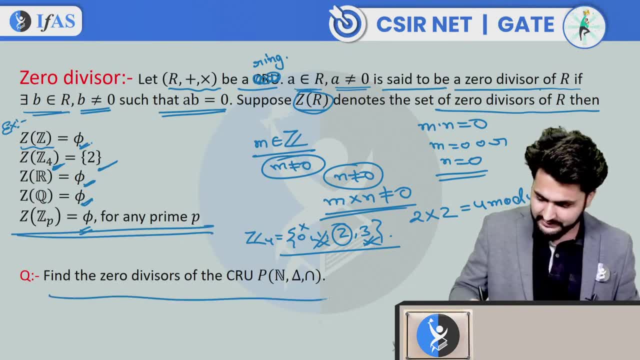 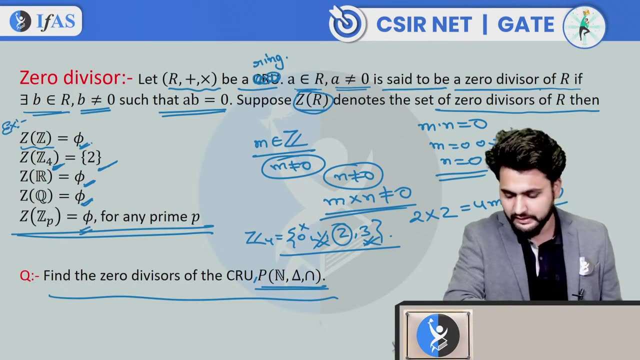 there is no zero divisor there. Now, this is the same example where you told the unit for power set of natural number element. So in this scenario, you will tell me that what is the power set of natural number with symmetric difference and intersection operation? 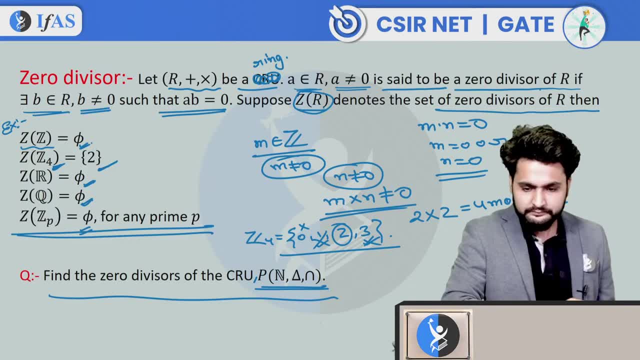 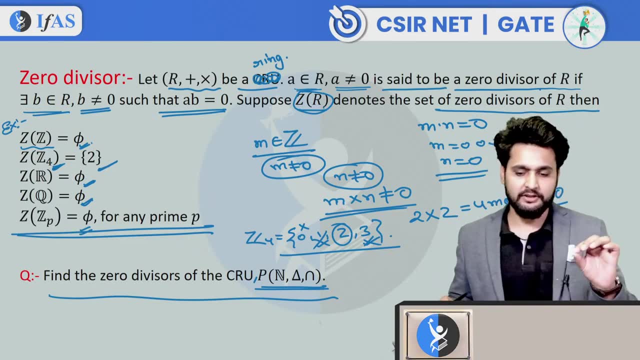 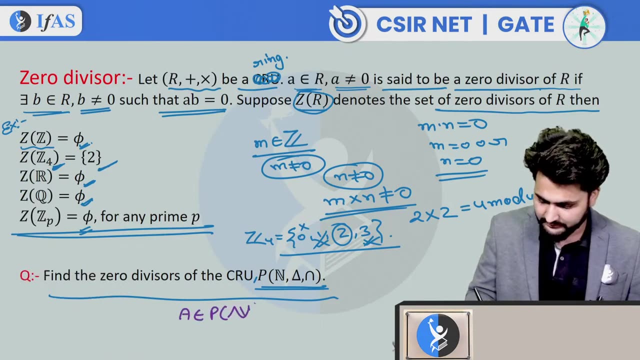 What do you think is the power set of natural number with symmetric difference and intersection operation? If I take any subset of natural number, let's say A belongs to power set of natural number- then it is a subset. So when will it be zero divisor? 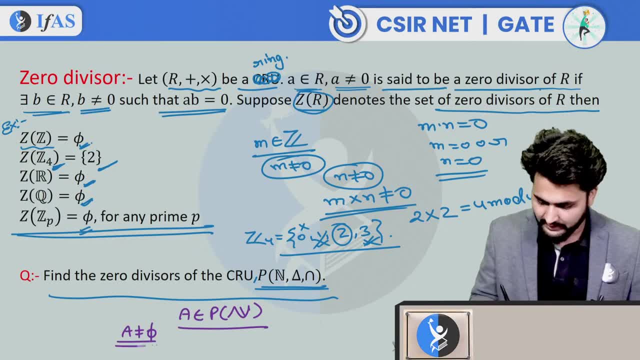 First of all, it should not be phi. A should not be equal to phi, It should not be phi, it should be non-empty. So if I assume that A is non-empty, then if I give the intersection of A to someone, 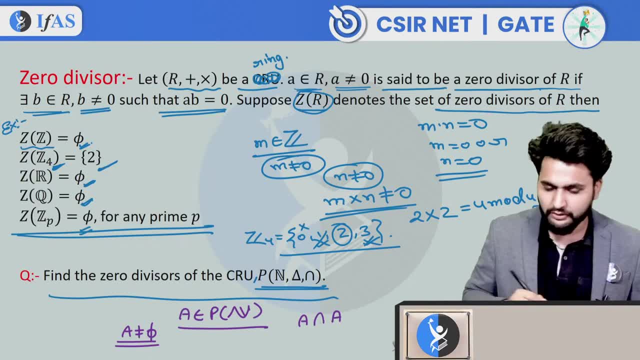 second operation. right, I can get another one so that it becomes zero. If I consider A as a complement, then how will it be? Neither it will be equal to n, nor it will be phi, because it is not phi And A should not be equal to phi. 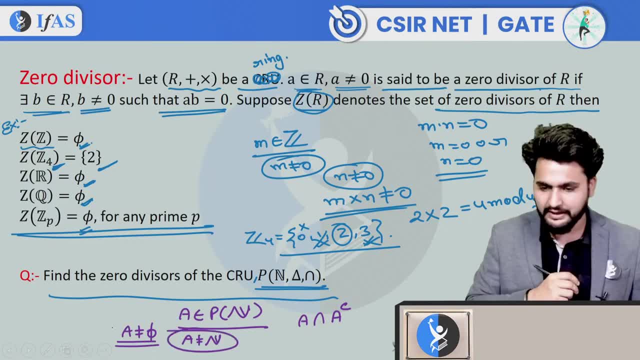 And also note that A is not equal to n. it is not equal to n either. So if you leave phi and n itself, then when you take out A as a complement, then A as a complement can neither be phi nor n. 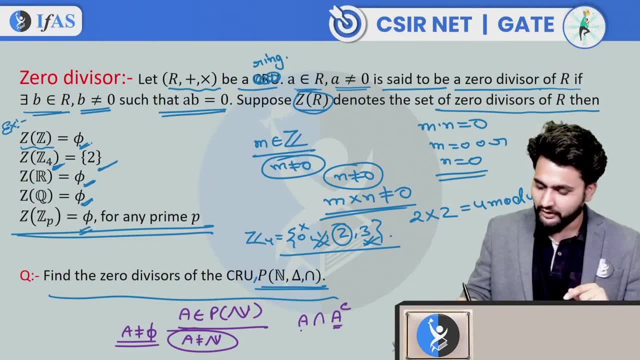 Why can't it be phi? Because there is no n, And why can't it be phi? Because there is no n, And why can't it be n? Because there is no phi. So A as a complement is neither phi nor n. 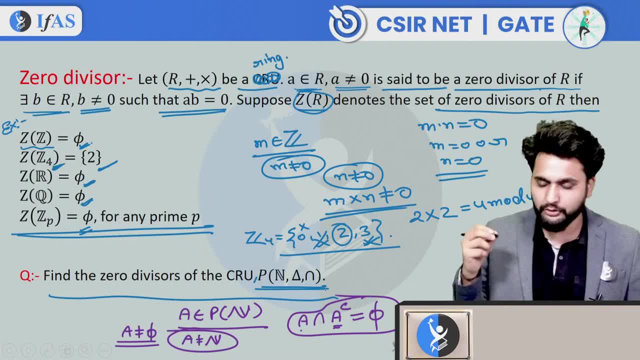 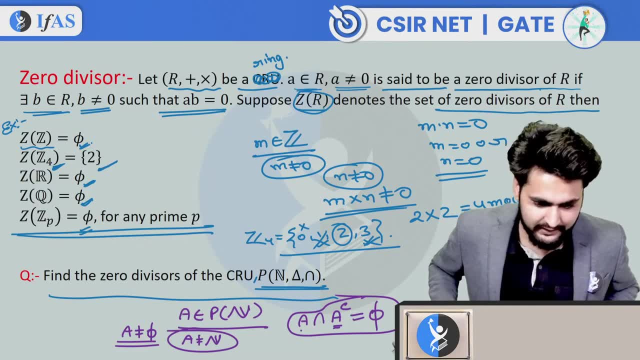 What will you get by complementing A? as a complement, You will get phi, which is a zero element of the power set of natural number Right. So n minus A, any proper non-trivial subset of n is a zero-divisor. 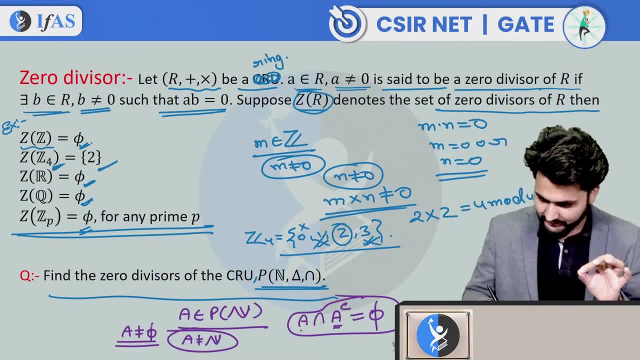 Perfect right. So any non-trivial- non-trivial means apart from phi, proper means apart from n. If you consider any subset, then it will be a zero-divisor only Because A as a complement is always equal to phi. 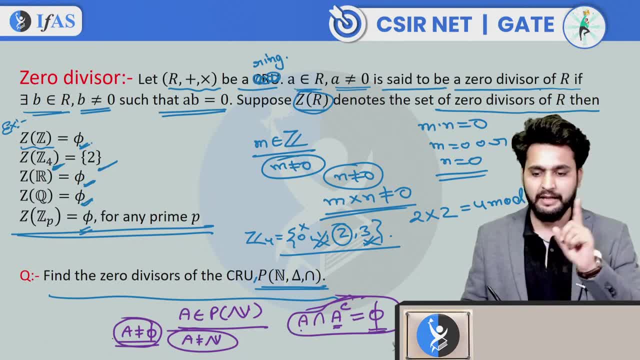 A is also neither equal to zero element nor n. A, as a complement, is neither equal to phi nor n. Both are non-zero elements. When you do product, product means when you do second operation, zero element means what? What will be the zero element of power set of natural number? 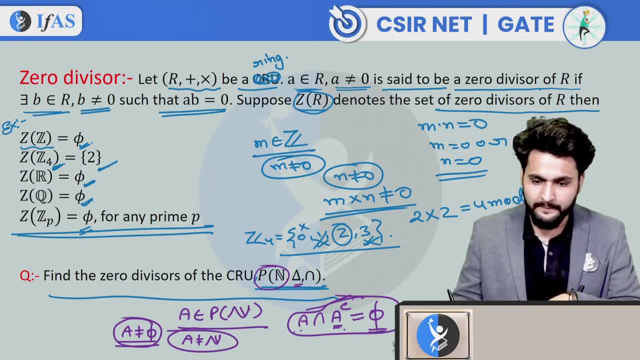 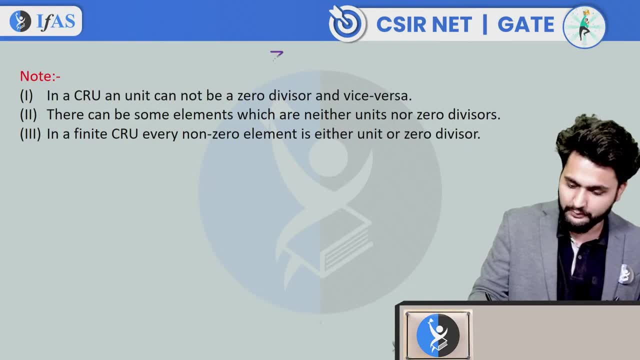 With respect to second operation identity element, which is phi. So all elements are zero-divisors. So if you want to write, you can write like this. We will see this note later. Z, if I ask you, power set of natural number. 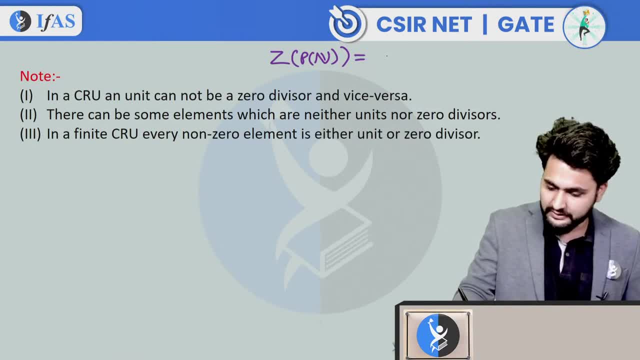 The collection of all the zero-divisors. What will be the power set of natural number? The whole power set of natural number will be there. Out of that, take out two elements. Take out one phi and take out one n. Apart from that, all are zero-divisors. 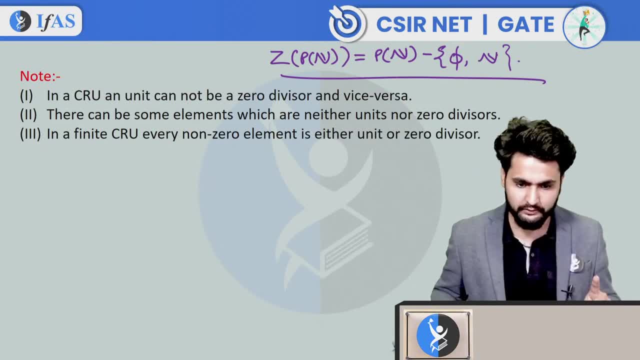 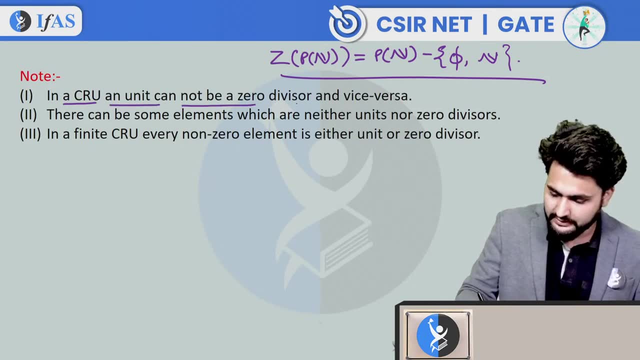 If anyone has any confusion, you can ask. Now there are some points to note down. The first point is: in a CRU, a unit cannot be a zero-divisor and vice versa In any CRU, not even CRU. 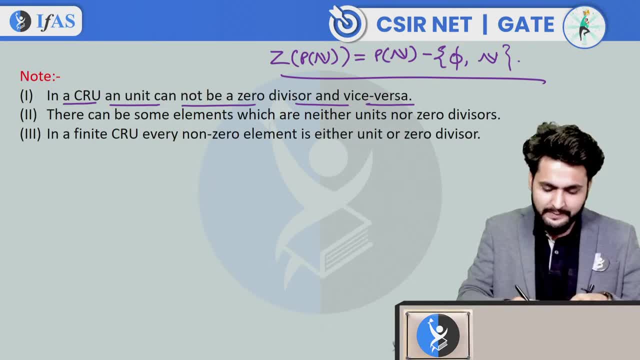 In CRU most of the time we stay in CRU. In this you can replace any ring In any ring. a unit cannot be a zero-divisor and vice versa. Unit cannot be a zero-divisor. Zero-divisor cannot be a unit element. 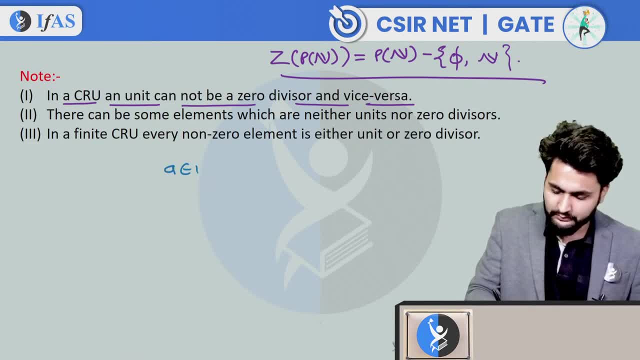 It can be verified very easily. Let's say I take a ring. Let's say A belongs to R And I have assumed that it is a unit and a zero-divisor. If it is a unit, then there exists. A' belongs to R. 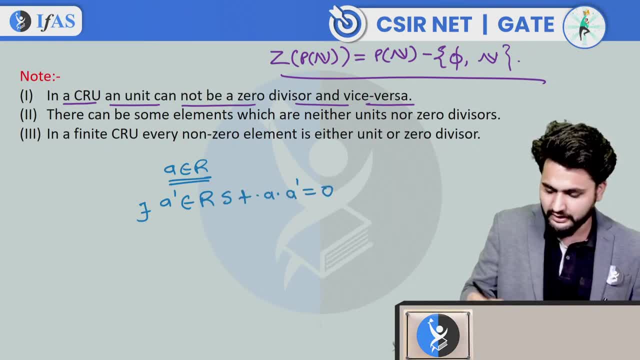 Such that A into A' is equal to unit element 1.. And if it is a zero-divisor, then what will it mean? There exists, let me say there exists, B belongs to R And A will be non-zero. 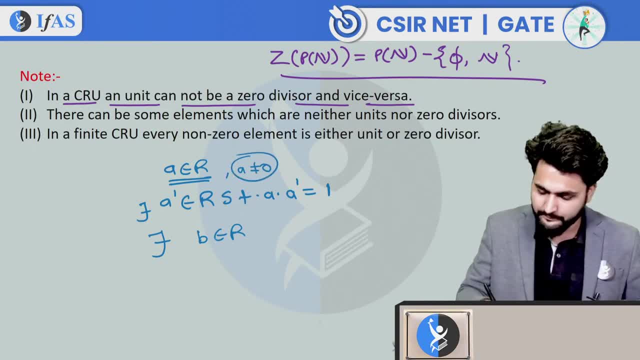 First of all, this unit, or any of the zero-divisors, will be non-zero. Right B belongs to R, Such that B not equals to zero. What will you get after doing A into B Zero? If it is a zero-divisor, then you will get another non-zero. 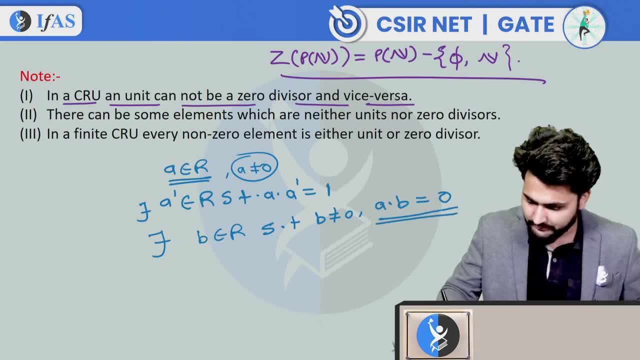 So what will you get after doing its product Zero? Now in this equation, if I multiply A' on both sides, So A' into AB is equal to A' into zero, Which implies that if you do A' and A nearby, then it becomes 1.. 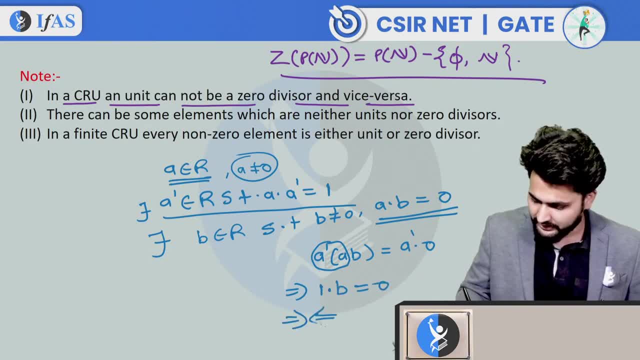 1 into B is equal to zero, And which is a contradiction to the fact that B is not equal to zero. We have considered this. So why is this contradiction being there? Because you have taken unit and zero-divisor together. 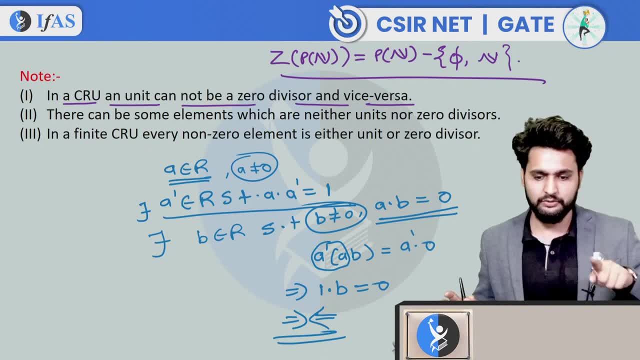 So they can never be together. If it is a unit, then zero-divisor will not be there. If it is a zero-divisor, then unit element will not be there, Right? So you have to remember this point. Next point is: there can be some elements which are neither unit nor a zero-divisor. 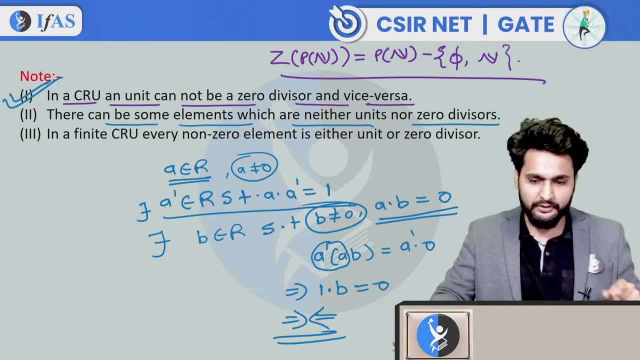 If you take any element, if it is a unit, then zero-divisor will not be there. If it is a zero-divisor, then it will not be a unit. But some elements can be like this: Not only a unit but also a zero-divisor. 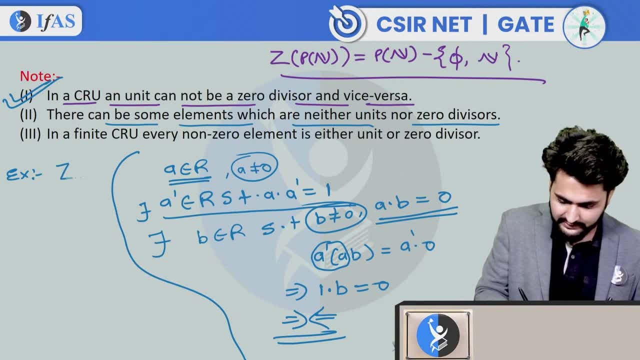 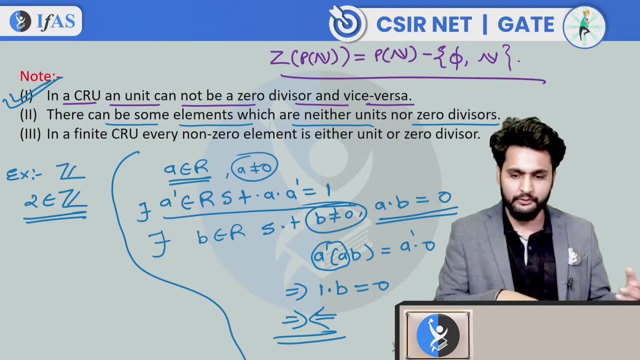 For example, if I consider z, let's say 2 belongs to z. Now tell me, is 2 a zero divisor? No, because 2 is a non-zero element and z does not have a zero divisor. So 2 is not a non-zero divisor. 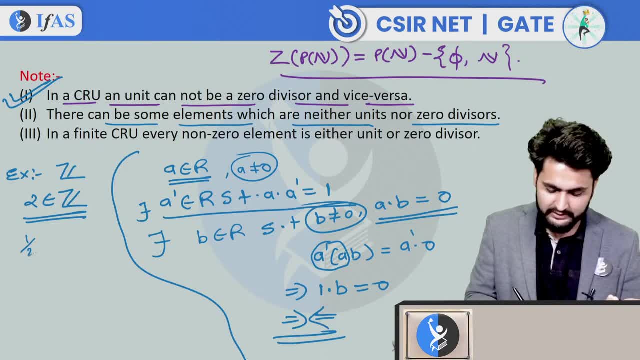 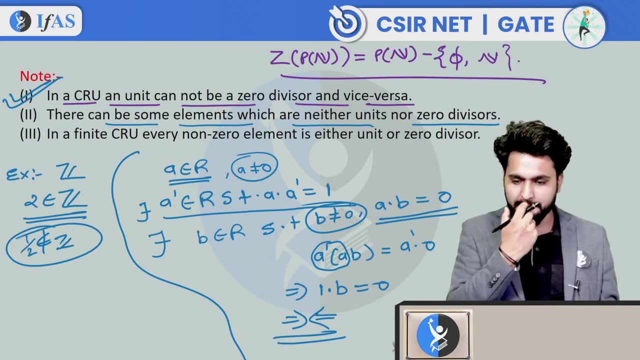 Is it a unit element? No, it is not a unit element, Because its inverse is 1 upon 2, which is not inside z. So there can be some element which is neither a unit element nor a zero divisor. So we can say something about rings, about when a unit element will be and when a zero divisor will be. 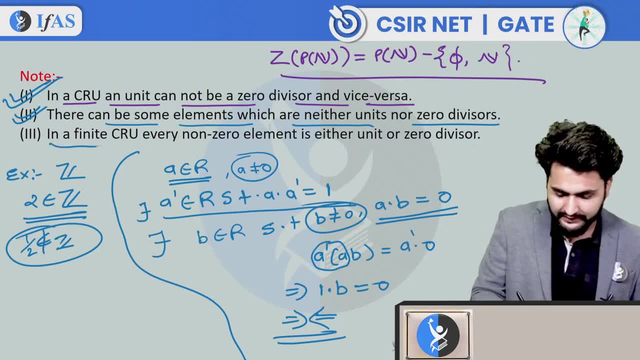 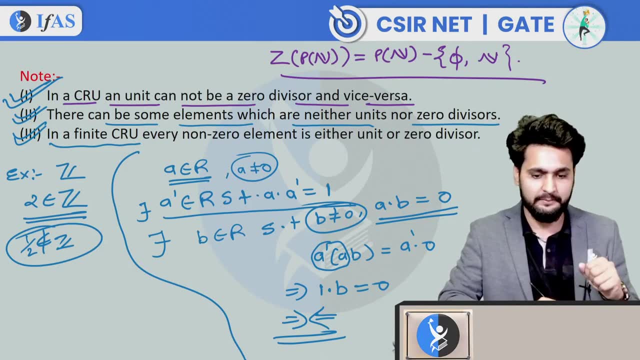 So this is our third point. The third point is in a finite CRU. this is a very important point. The third point helps you in many proofs. I will tell you in one proof how you can use it. In a finite CRU, every non-zero element is either a unit or a zero divisor. 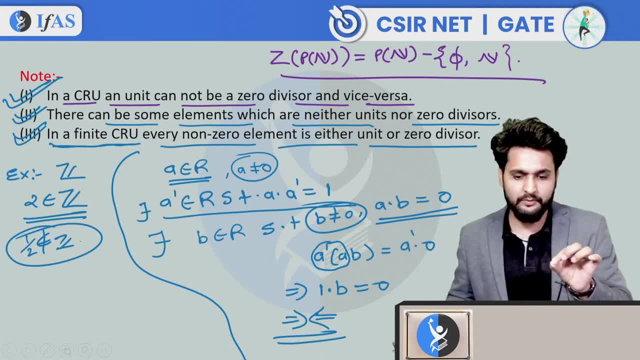 So the element which you have got in z is neither a unit nor a zero divisor. This can never happen in a finite CRU. If there is a finite CRU, if you take a finite commutative ring with unity, every non-zero element of it is either a unit or a zero divisor. 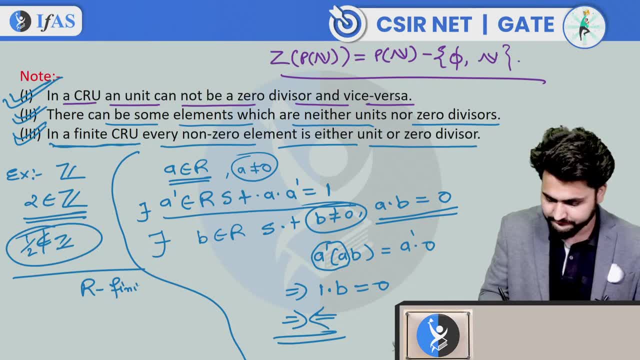 For example, I have taken R. How is this? This is a finite CRU, A finite commutative ring with unity. Let me consider: A belongs to R. A0 equals to 0.. I have considered a non-zero element. 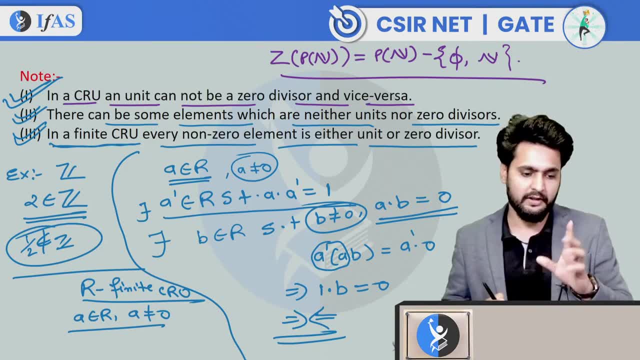 As you have taken this, either it is a unit or a zero divisor for sure. It is not possible that you have got it in z, neither a unit nor a zero divisor. So in a finite CRU this is not possible and we get a lot of benefit out of it. 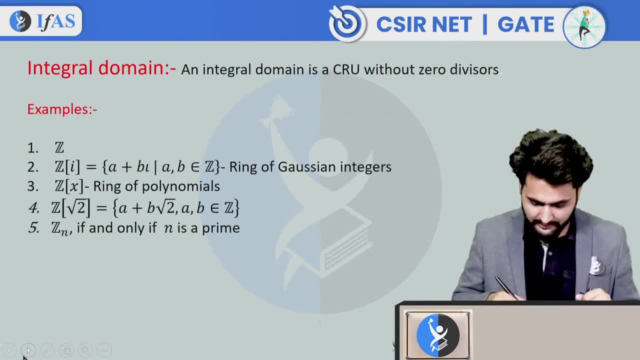 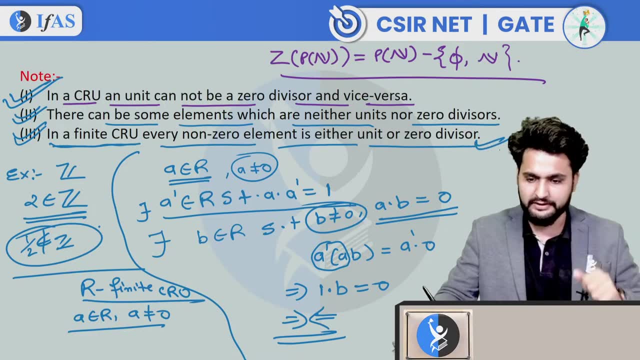 Let us understand how we get the benefit. Let us define the integral domain first. After defining the integral domain, I will show you how we can use it many times. For example, you have to find the number of zero divisors in zn. 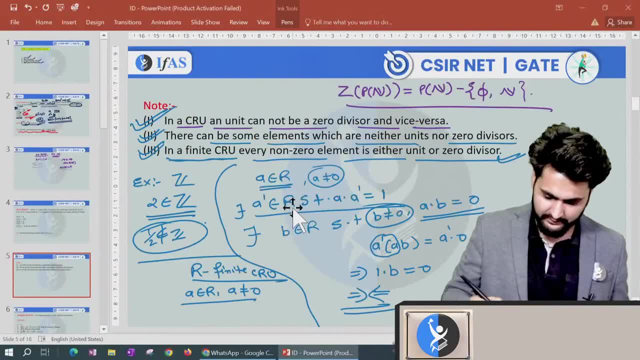 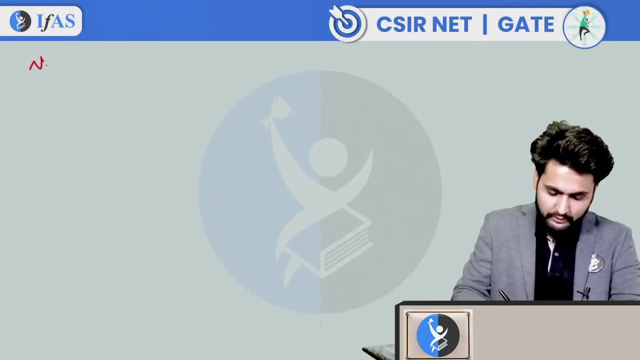 So you can use it here. Give me a second, I will add a page. For example, if I ask you how many zero divisors are there in zn, Someone would like to tell Number of zero divisors of zn? 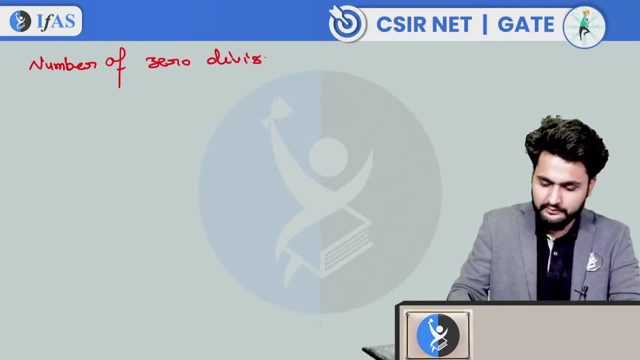 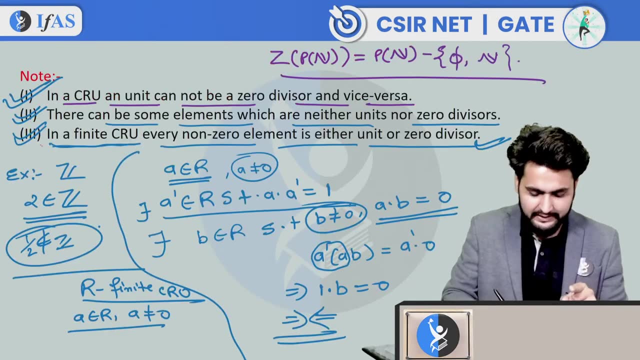 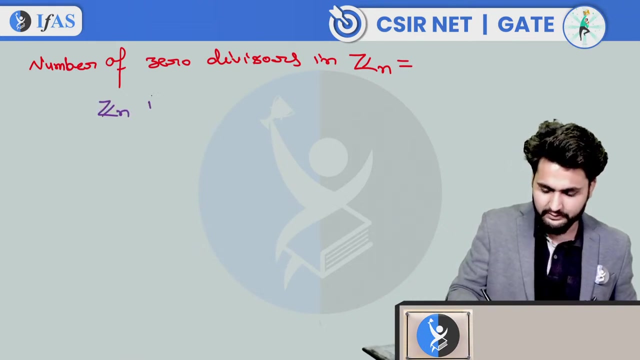 Number of zero divisors in zn. How many zero divisors are there in zn? Someone would like to tell? Now, if you use the last point I have written, you can get it easily Why? Because we know in zn that zn is a finite CRU. 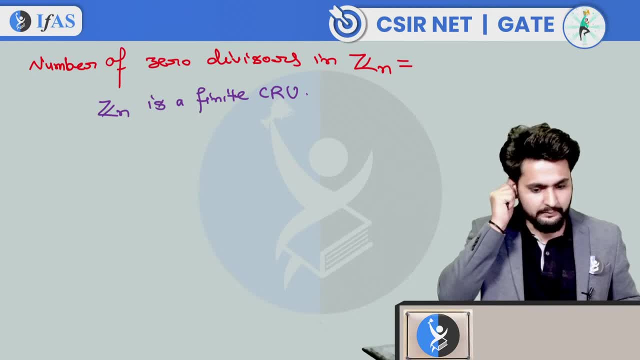 It is finite. Number of elements is finite. Commutative ring is also there. Multiplication is also commutative. Unity is also there. So finite CRU. Unity means that one always stays in it. So this is CRU. 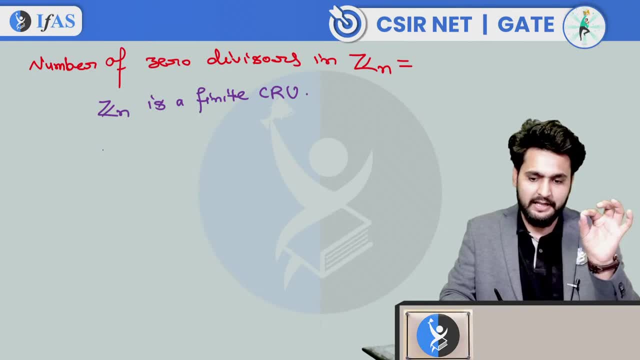 Fine, Now finite CRU. if you take any element of it, either it will be a unit or zero. divisor Every non-zero element. What is the total number of elements in zn? It is n. Out of this, if I take out zero elements, one element is zero. 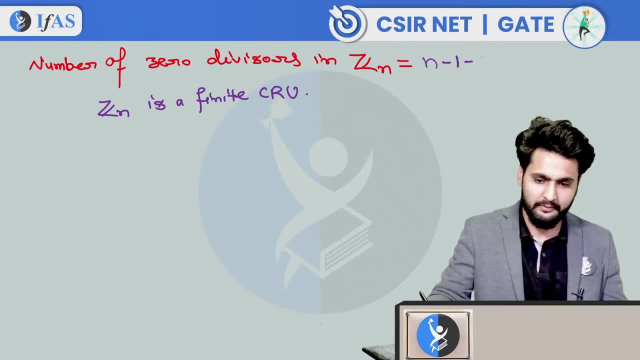 And if I take out all the unit elements, what will be left? It will be zero divisors. So I took out minus phi n. This is the formula for you. Apart from unit and zero, everything is correct. Right, So this is the formula: n minus 1, minus phi n. 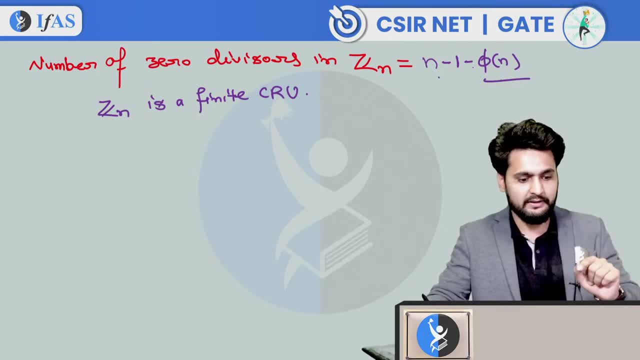 Is that clear to everyone? We can use it in this way. Now we will see one more result where we will say that in a finite- let me say every finite- integral domain is a field. So it is very helpful to verify that too. 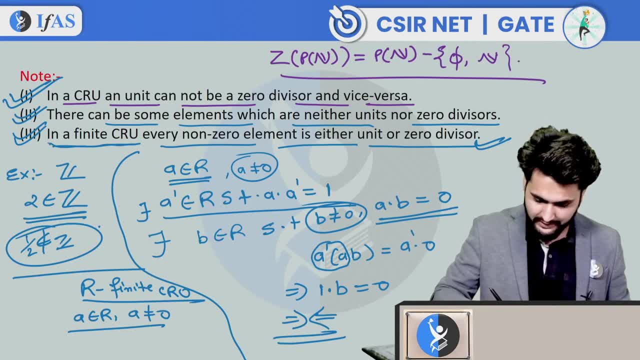 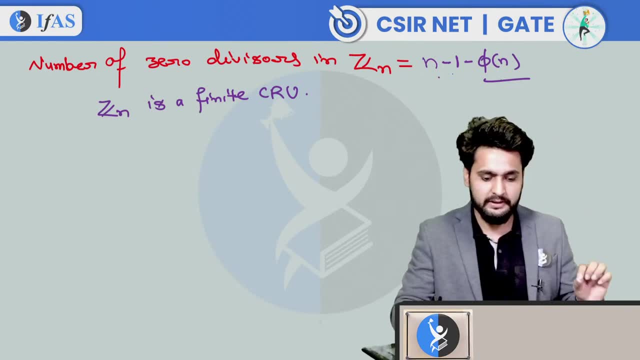 I will show you now, So you have to remember this point. It is very helpful for you many times. Okay, So what did you understand from here? Number of zero divisors in zn is equal to n minus 1 minus phi n. 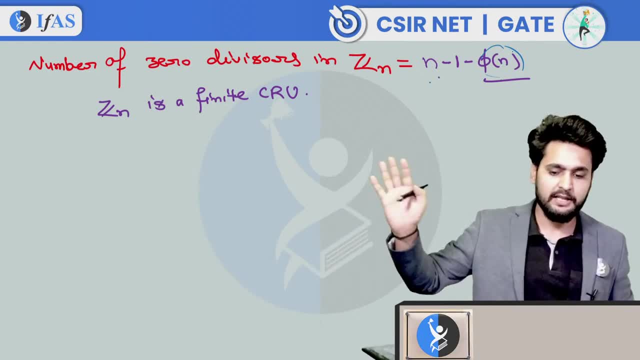 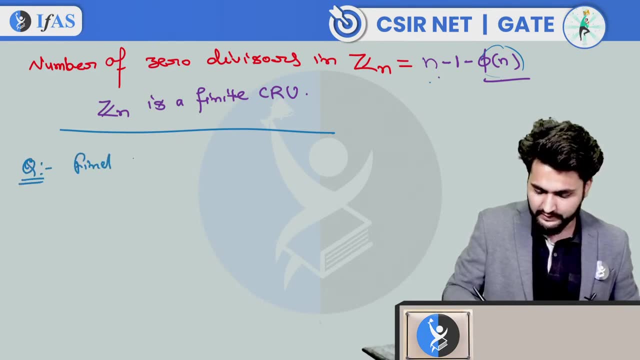 Because there are so many unit elements. I took out the unit, I took out zero. So what will be left? All of them are zero divisors. So just tell me one question. Let me ask you: Find the number of zero divisors in z100.. 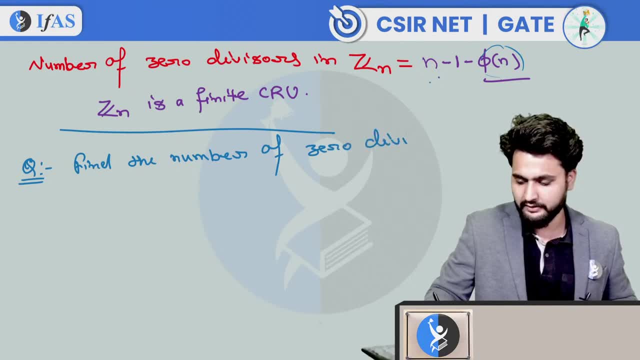 Number of zero divisors in z100.. In z100.. In z100, how many zero divisors will be there in total? Just tell me by taking it out, Anybody? Yes, Yes, Yes. Let me ask you another question. 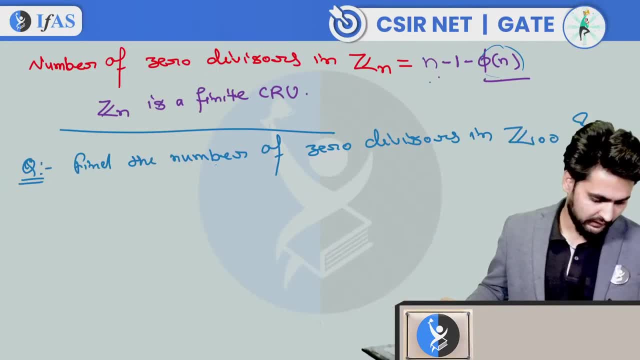 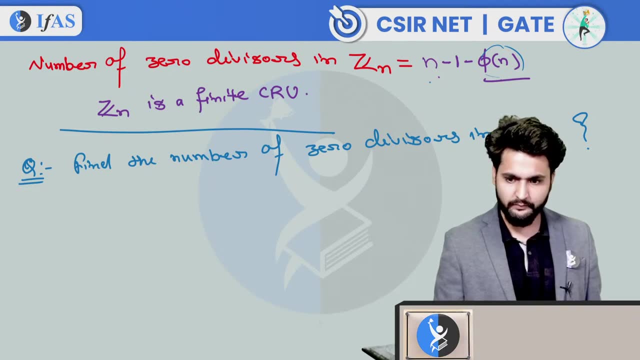 How many resources will it have in z100?? What do you think? Look for it and give me your answer. After that we will learn about integral domain and its properties. number of zero divisors in z hundred: z hundred mein total kitane zero divisors hota hai can. 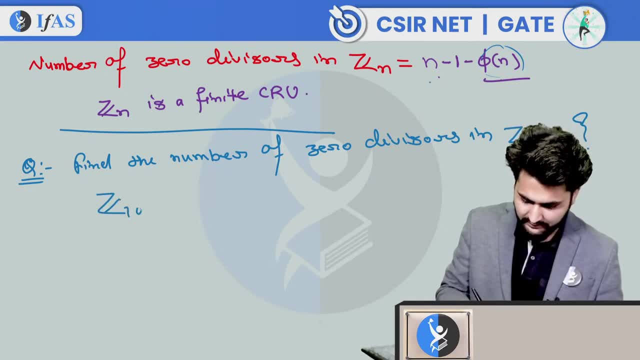 you find this? apko upar formula likha hua dikh raha hai. toh mujhe nahi lagta, isme kisi ko bhi problem hona chahiye. jaldi se iska answer karo. what do you think? number of zero. 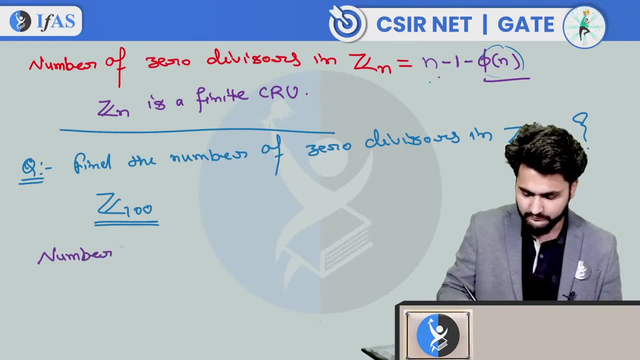 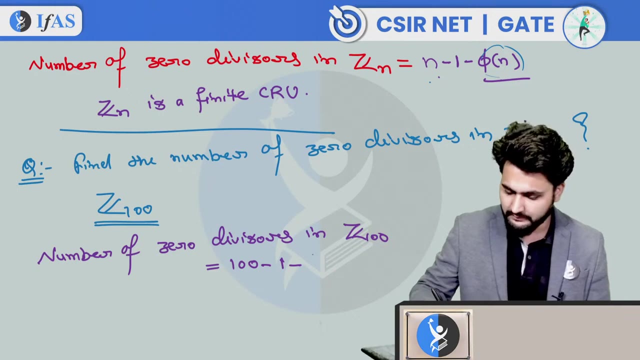 divisors in z hundred is equals to number of zero. divisors in z hundred is equals to hundred. mein se ek zero element nikal diya, aur zero element ke baad mein five hundred, jo unit elements hai, wo bhi humne nikal diya. these are the 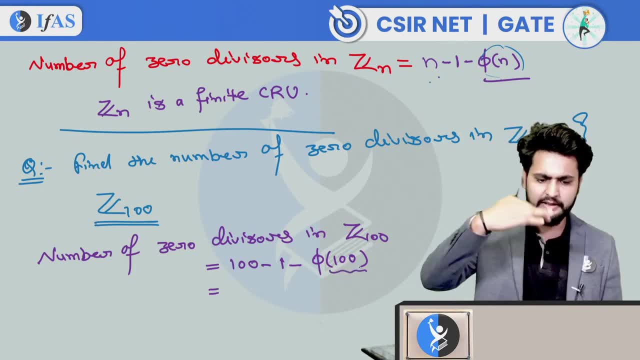 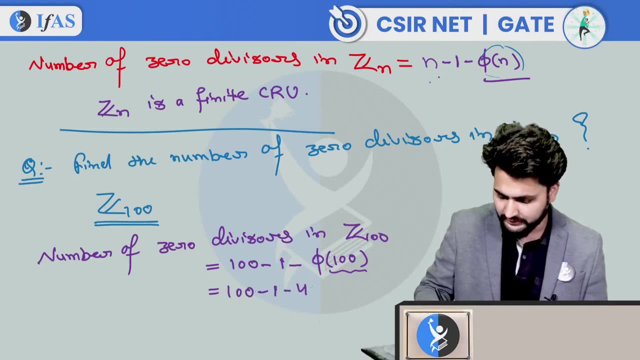 unit element- yeh aapko sabko pata hai. unit element, yeh un group jo banate ho, toh isle maine nahi likha hai. so this is equals to hundred minus one minus forty. yeh five hundred nikalna aapko aata hoga. absolutely correct, shayante and shabna. very good, right. so this? 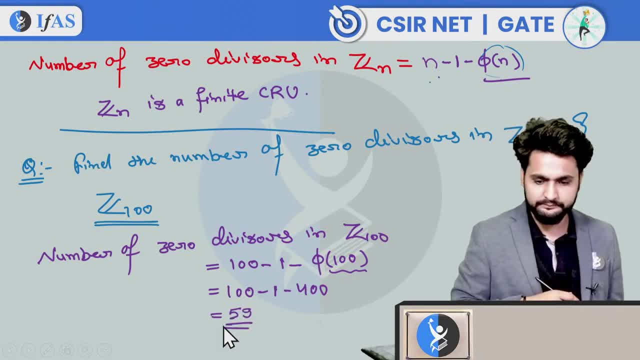 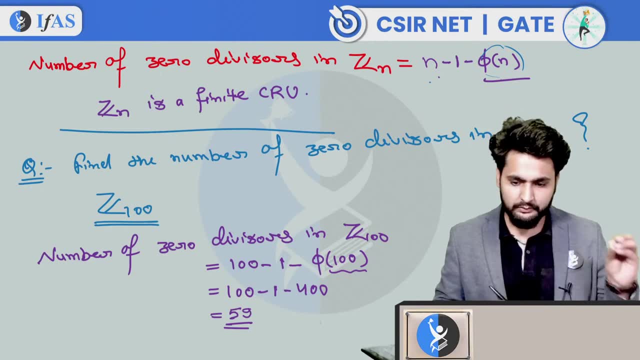 is fifty nine. yeh kitna jayega aapka. fifty nine, aapko aata hoga. absolutely correct, shayante and shabna. very good, right. so this is fifty nine and forty one aapko. kya mil jayega unit element aur zero hai. na hu milke. forty unit element. 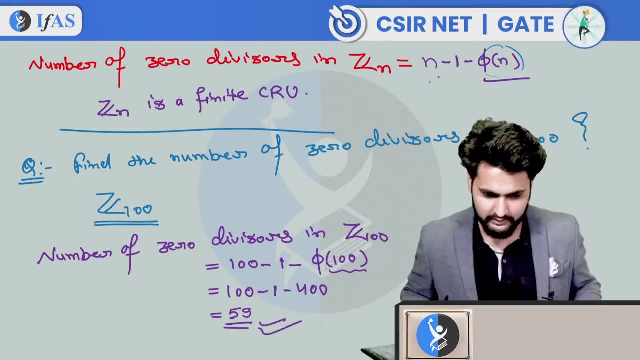 honge ek aapko zero aur nikal hoge, toh aapko kitna milenge: fifty nine, correct right, so fifty nine aapko zero divisors mil jayenge z hundred mein aap nikal chakte ho, aasaani. 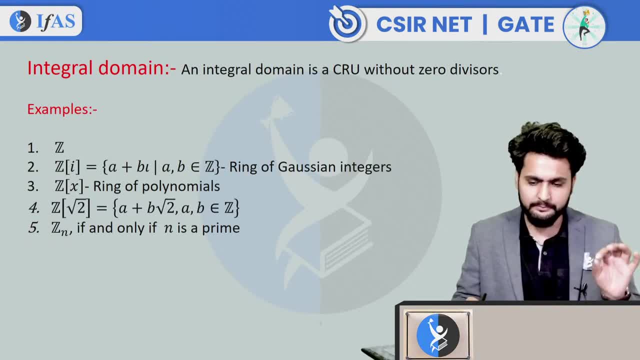 se thike. ab aage varte aur integral domain ki definition dikhte hai. kya hota hai simple definition integral domain ka koi bhi ring, agar commutative ring with unity hai, uske paas zero division nahi hai, toh integral domain hai. ek chich dhaan raki, yeh bhi jaroori. 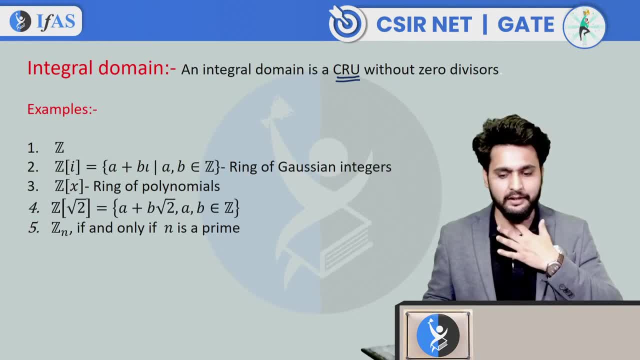 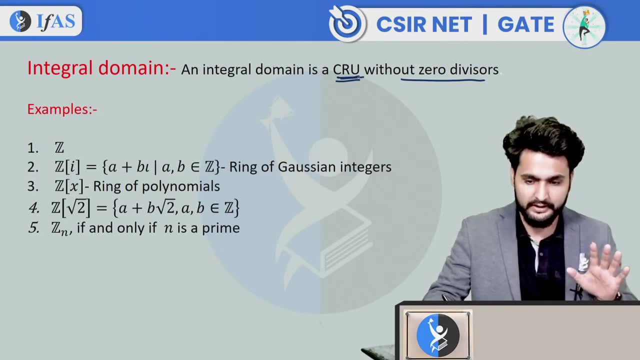 yeh miss kar dete hai, as it correct, kai baar hum kya garte hai, hum keval zero division ka dhyan raktay, ki zero division nahi hone chahiye, toh integral domain ho jayega. par aisa nahi hai uske liye CRU bhi hona chahiye. sabse pehle change hai an integral domain. 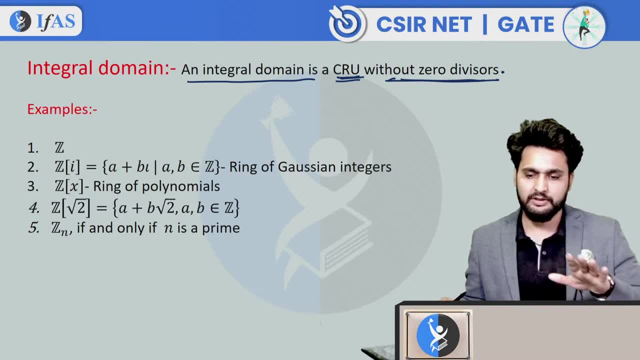 is a CRU without zero division. koi bhi CRU, jiske paas zero division nahi hai, wo integral domain hai. agar CRU nahi hai, tbhi integral domain nahi hoga. agar ek bhi uske paas zero divisor hai, tbhi wo integral domain nahi hoga. jaise, sabse pehla example aapko dikh raha. 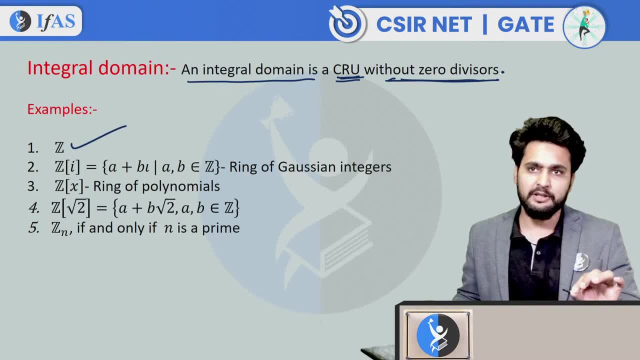 hoga. z it is an integral domain. a integral domain hai commutative ring with unity hai koi bhi element, zero division nahi hota hai. toh iska matlab kya hoge. integral domain. z? i is an integral domain, ek bhi element. 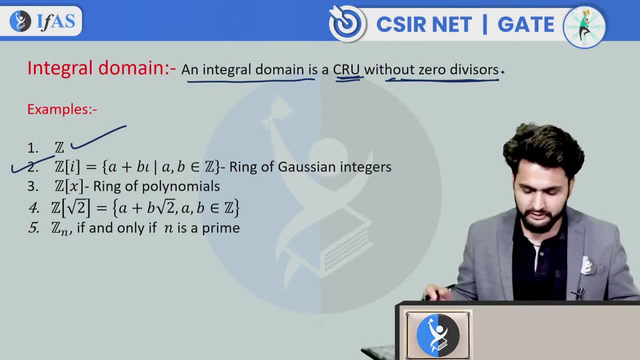 zero division. nahi hai uske alaba CRU, toh hai usme koi issue nahi hai. z x is an integral domain. infact, agar polynomial ring aapne padha hai vise, toh mai aapko padhane wala ho issi. 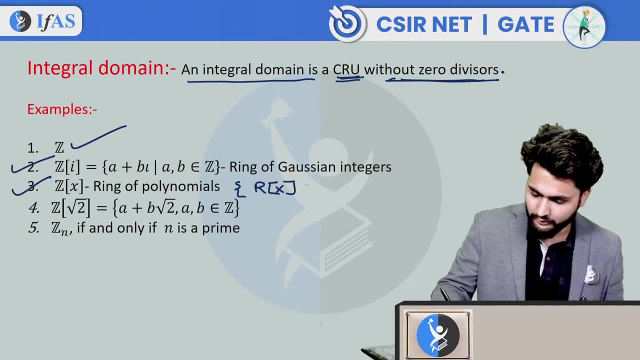 week me polynomial ring. bhi r x is a integral domain. is integral domain if r is a, not if, if and only if r is an integral domain integral domain. r is an integral domain hai, toh r x bhi integral domain hoga, r x agar integral. 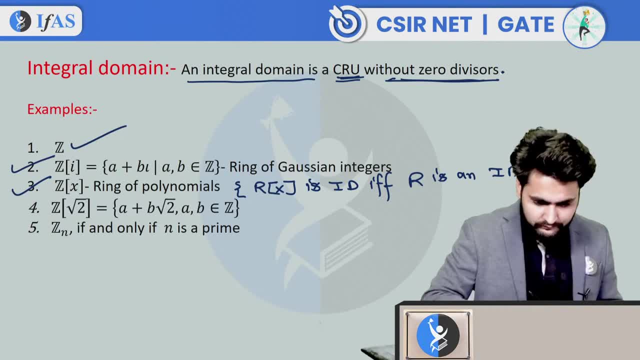 domain hai, toh r aapka integral domain hoga. manassha, it is correct: 100 minus 41, is that? ok, toh ye integral domain hai. this is also an integral domain. ye bhi integral domain hai. z? n is integral domain if, and only if, n. 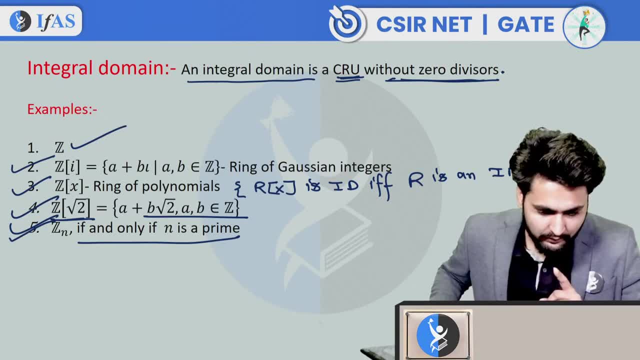 is prime z n integral domain. tabhi hoga ha bilkul mine ideal. ha aapka shayanta maine comment dekha, tab sayad maine padh nahi paaya aapka comment bilkul maine aapka comment bhi. 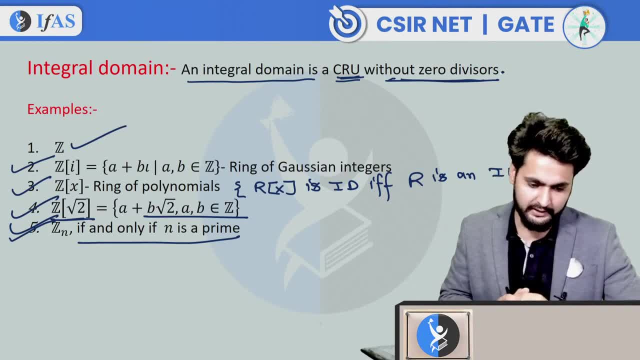 dekha hai. if possible, toh jitna jaldi hoga, mai video bana dunga aapke liye. fine, acha question bhi aapka, acha aapne uske baare me socha bilkul hum uspe baat kar sakte hai, ki under homomorphism 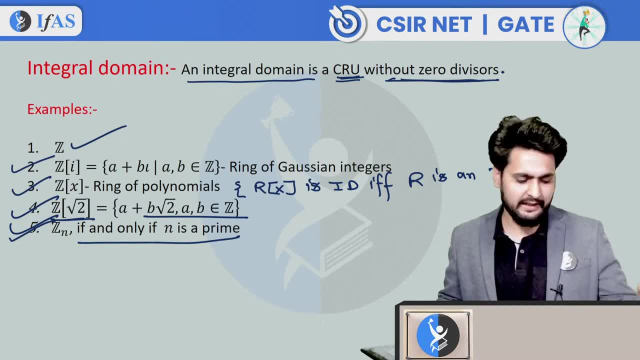 kya hota hai, right, prime, prime pe map karega, ideal, ideal pe map karega. kya conditions ho sakte un sab pe baat kar sakte hai tike, toh, jaisi possible hoga, mai video uspe bana dunga. 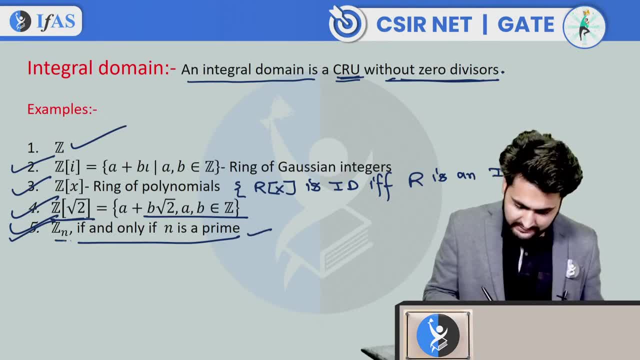 fine, ok, toh ye saare aapke kya integral domain hai. ek chiji ye dhaanak, ye z n is a z n integral domain? kab hoga hai? if, and only if n is prime. agar n prime nahi hai, toh hum kai baar sath. 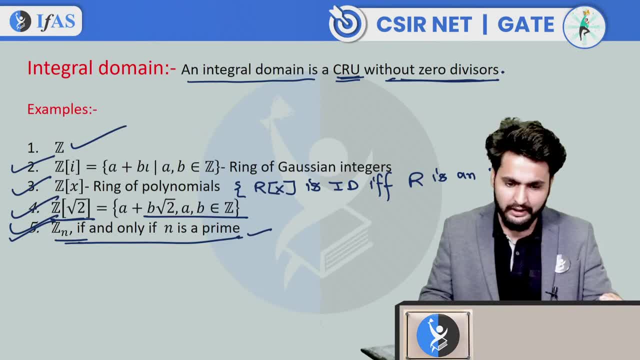 baat bhi ka chukiye: agar n prime nahi hai, toh uske baar zero divisors hoga, hala ki c r u hoga. agar n prime nahi hai, toh for sure uske baar zero divisors. humge kyu kyunki. 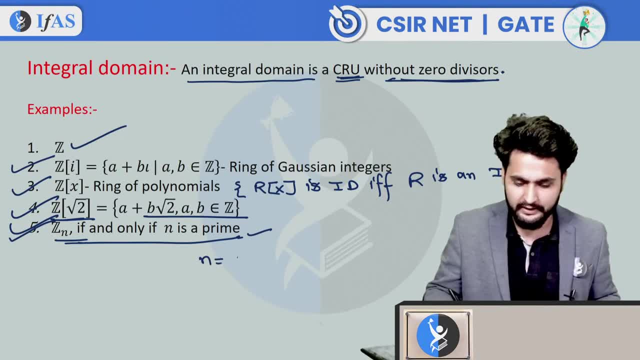 agar let say n prime nahi hai, toh kamsa, kya 2 factor, toh uske baar humge. let say p and q maal liya factors hai. so jaisi ka p aur q logi, ye dhunon non zero element hai z n. 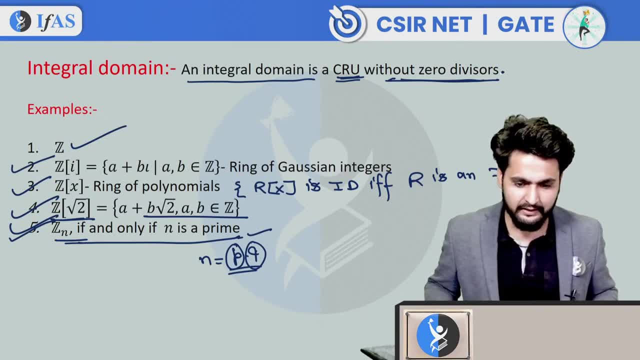 ke element hai, inka product karne par aapko kya mil jayega zero mil jayega kyunki p into kyu karoge, toh n ke barabar hi hoga. apko zero divisor dedega. so z n is an integral. 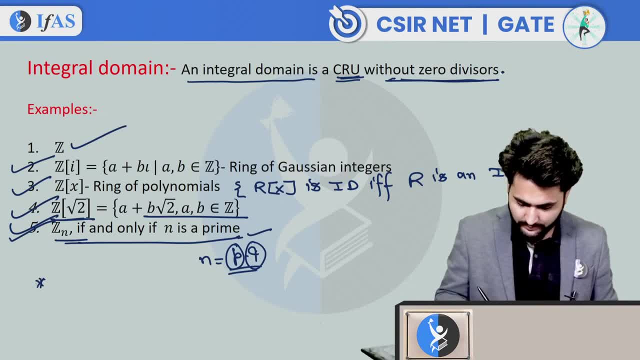 domain if, and only if, n is prime. baaki aap ye bhi likh sakte ho: every field is an integral domain. hai bhi ek example uskta hai: every field is an integral domain is an integral domain. ab isme kuch verify karna hai. 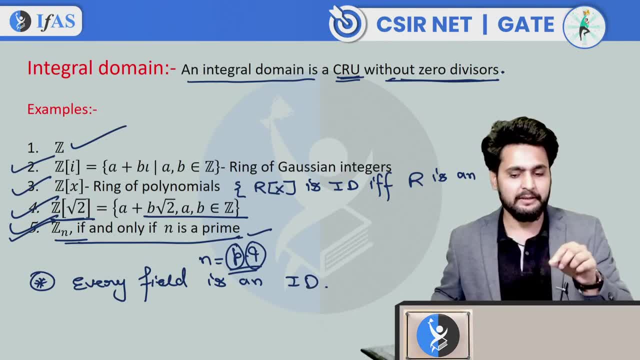 field me har ek non zero element kya sath unit hota hai. jab har ek non zero unit hai, toh zero divisor. toh ho nahi skta iske matluk: kya hogia integral domain? hogia, so every field is also an integral domain. these are some examples ume de apko definition. 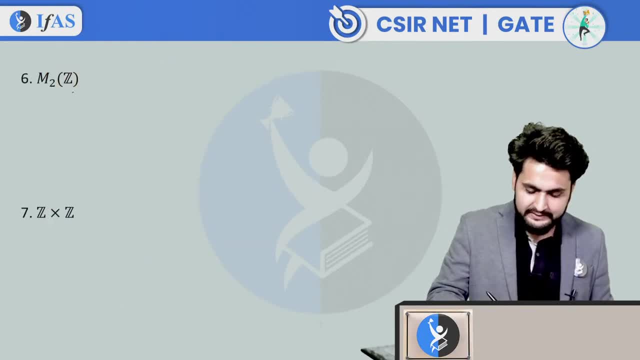 clear hoga: integral domain: kya hota hai kuch? ek aur example: dekhte jaise z cross z apko dekhte hai? z cross z apko dekhte hai this is: is this an integral domain? let me ask you. 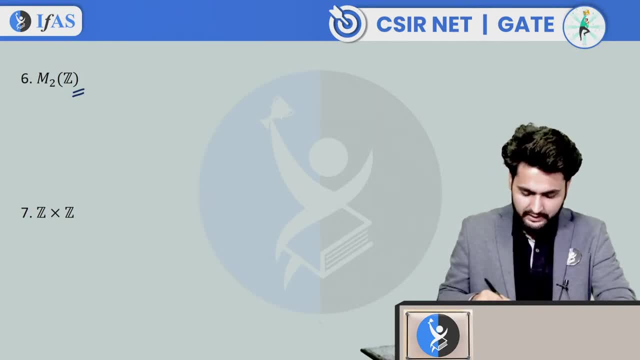 6 number pe jo aapko dikh raha hai. kya ye integral domain hai. batao ki chalo 6z jo aapko dikh raha hai. 6 me aapko dikh raha hai. sorry, m2z. 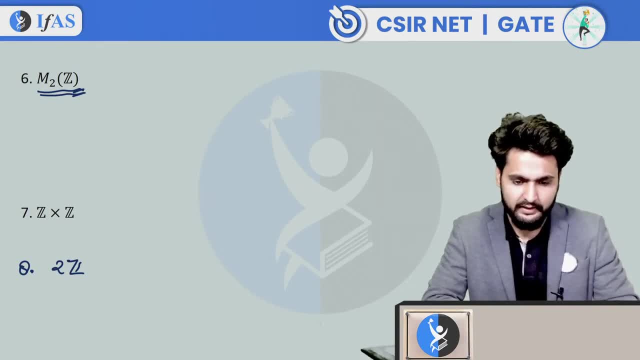 is it an integral domain? kya ye integral domain hai? m2z- is it an integral domain? ye CRU hai. commutative multiplication hota hai. kya pehle thing to ye CRU hi nahi hai. this is not a CRU, not a CRU. 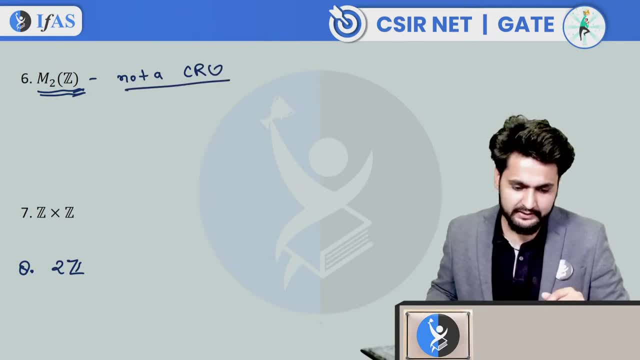 commutativity hi nahi hai to ye integral domain. kaise ban sakta? pehle cheez hai, aur iske paas. zero divisor bhi hai, shanti, you right. zero divisor bhi hai, iske paas, agar main let's say 1, 0, 0, 0. 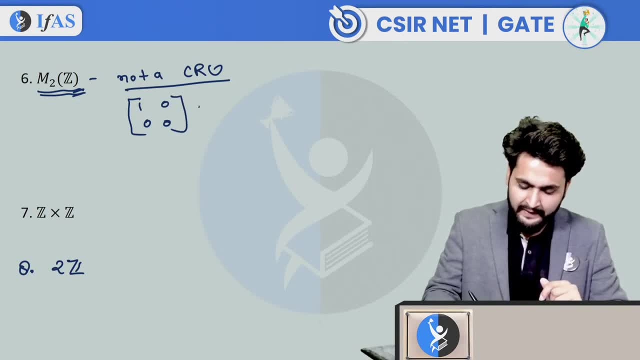 ye, ek matrix le liya- this is a non-zero matrix, correct, shabna right- and ek dusra le liya. let's say 0 0 0, 1. these both are non-zero elements of m2z aur jaise inka product karoge. 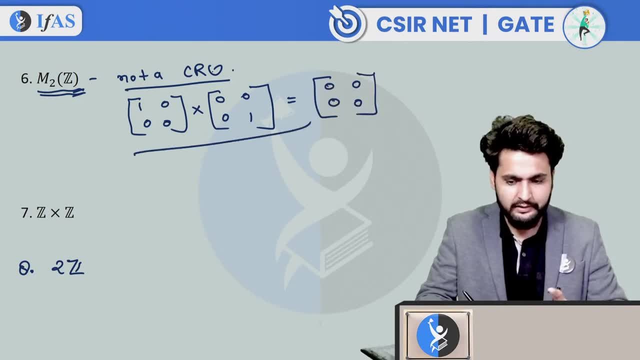 0, 0, 0, 0 mil jayega to ek to ye CRU. nahi hai dusri cheza iske paas zero divisor bhi hai to integral domain. ho hi nahi sakta. this is not an integral domain, if i ask you. 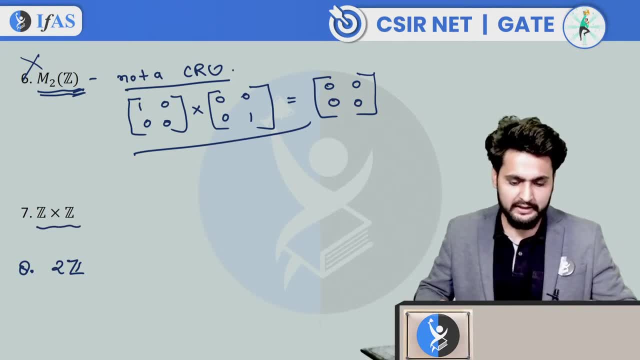 z z z cross z. kya ye integral domain hai? ye bhi integral domain nahi hai? kyunki iske paas, agar main loom 1 comma 0 and 0 comma 1 element, ye dono non-zero element hai. is ring ke. 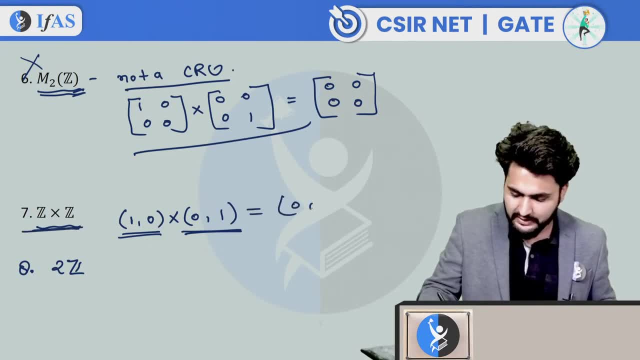 aise hi to element dikhengi hai aur inka product karne par, aapko kya mil jayega, 0 comma, 0 mil jayega, in fact. in fact, aap kya bol sakte ho ki i1, cross, i2. 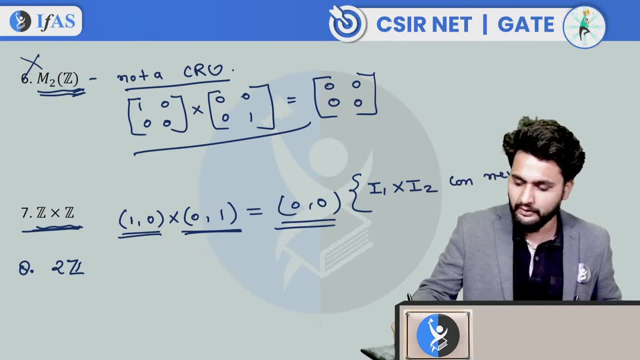 can never be an integral domain, can never be an integral domain, integral domain where, let me say, where i1 cross i2, where i1 and i2 are integral domain, where i1 and i2 are integral domain. agar 2 integral domain, aapke paas hai. 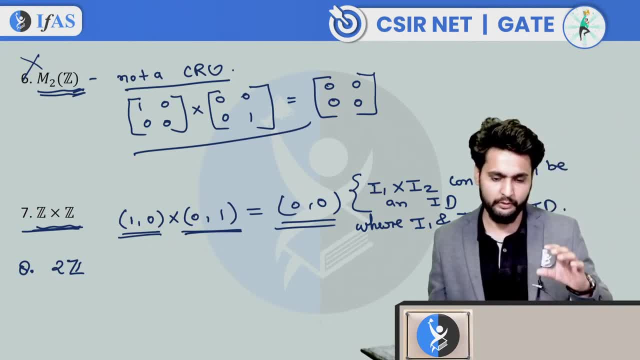 to unka cross product kabhi bhi integral domain nahi hoga. 2 integral domain ka cross product kabhi bhi integral domain kyunki. kyunki, agar integral domain hai, to CRU hoga. i1, i2, kaise hongi? 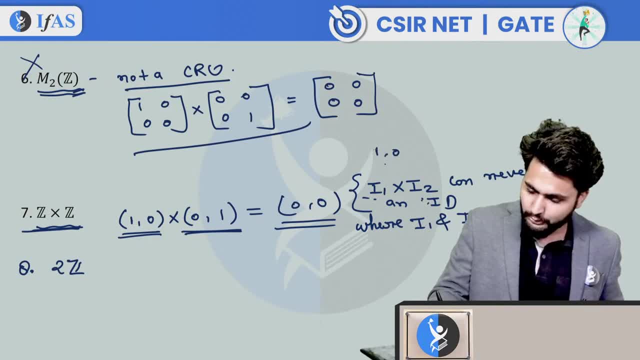 CRU uske paas 1 hoga to yaha. se aap ban loo, yaha se 0 lele 1 a element mil gaya 2 element. kya kar aapki baar yaha se 0, 0 bhi hoga, hi hoga. 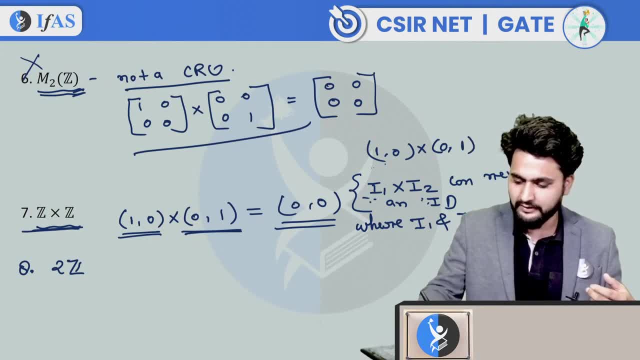 ring hai to 0 to hoga na right aur CRU hai to 1 hoga to idhar. se ban loo to ye hamesa 0 divisor hoga agar integral domain hai i1 i2 to i1 cross i2 me. 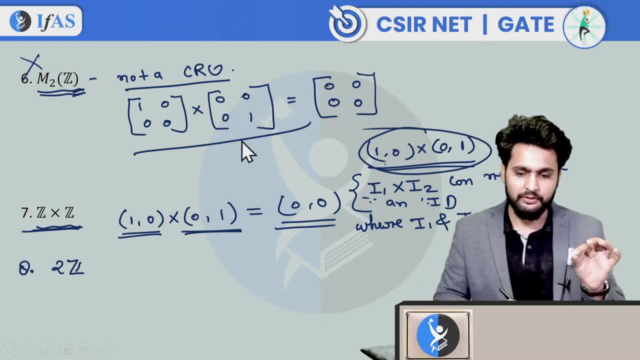 ye 0 divisor hamesa hi aapko milenge hai, na to 2 integral domain ka cross product. kabhi bhi integral domain nahi hota hai. let me ask you about this 2z ke baari ma aapse puchta ho. 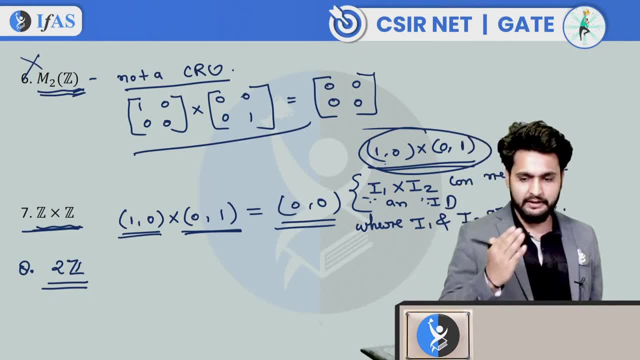 kya 2z ek integral domain hai. ek ring hai z ke anwer contain hota hai. sub ring hai z ka to khud mein. ek ring hai kya lakta hai: 2z is an integral domain or not? if i consider, let say: 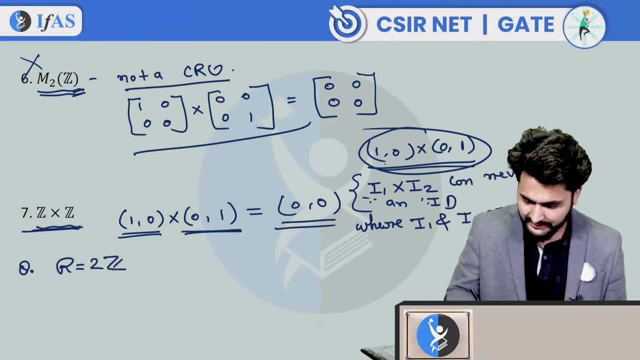 r is equals to 2z, kya ye integral domain hai. what do you think? kya ye integral domain hai? is r equals to 2z? is an integral domain. what do you think? 1 is not in 2z, so not. so this is not a. 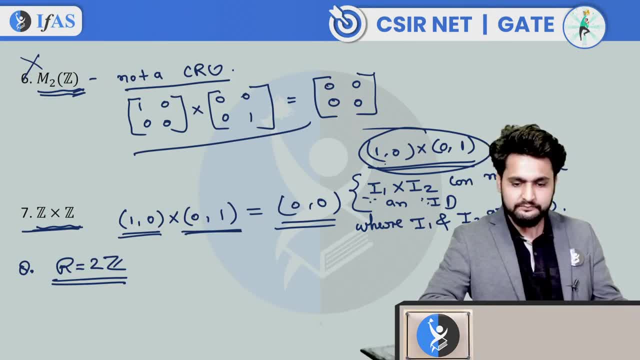 ring with unity. very good, shanta right, it is correct. isme kai baar confusion hota hai, aur kuch log to even isko maante bhi, kuch authors isko consider bhi kar leta integral domain, but jo ham log padte hai. 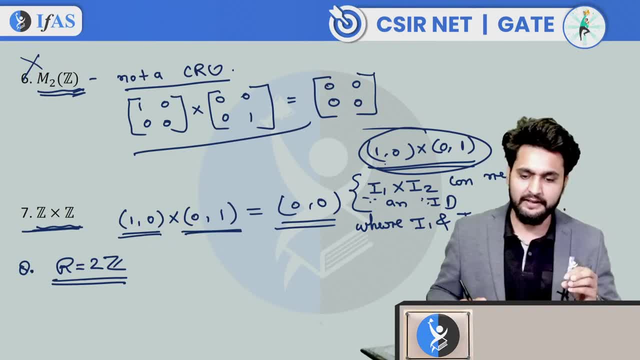 waha pe apne ko isko integral domain nahi maata, because 1 is not, this is not a CRU. not a CRU, not a ring with unity. agar apko aur precisely bol la hai, to aap kya bologe: this is not. 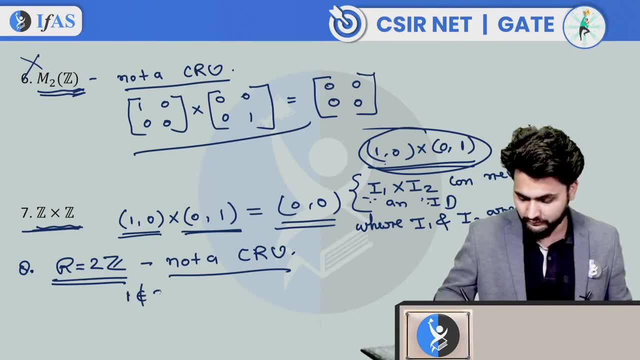 a ring with unity isme. 1 nahi hai. 1 not belongs to 2z isme. achi jeez ye hai ki koi bhi zero division nahi hai par unity element naa honi ki wajah se apan isko kya karenge. 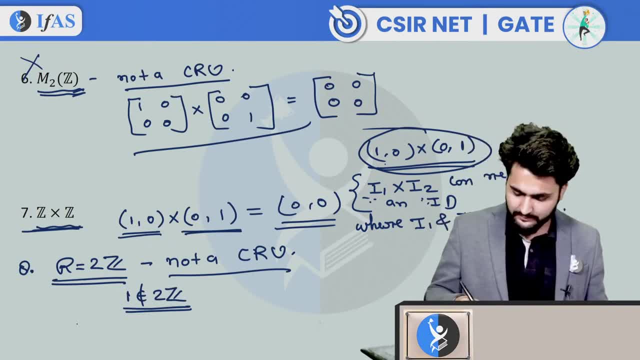 integral domain nahi bolte hai. is that clear to ek chich aur bhi aapko yaha, se aap kya kar sakte ho, aap likh sakte ho, ki mz is not an integral domain, isme is not an integral domain. 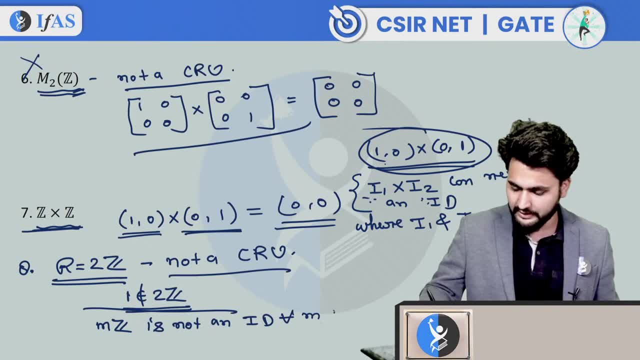 is not an integral domain, for all m belongs to z comma. m is not equals to 1 comma minus 1 mai idhar likh letao m is equals to 1 comma minus 1, 1 aur minus 1 ke alaba m ka. 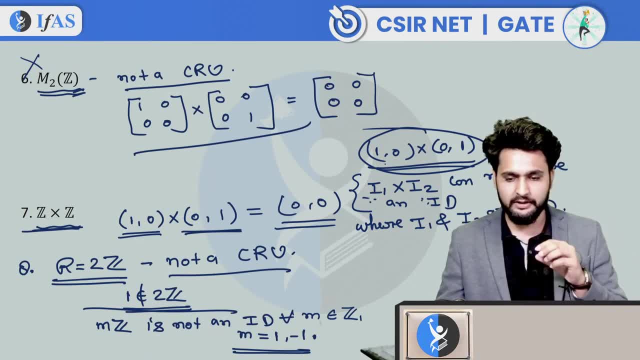 koi bhi value le liye. kabhi bhi mz integral domain nahi vane ga kyo kyunki. 1 minus 1 ke alaba. kuch bhi value aap doge to uske pas, 1 hoga hi nahi. 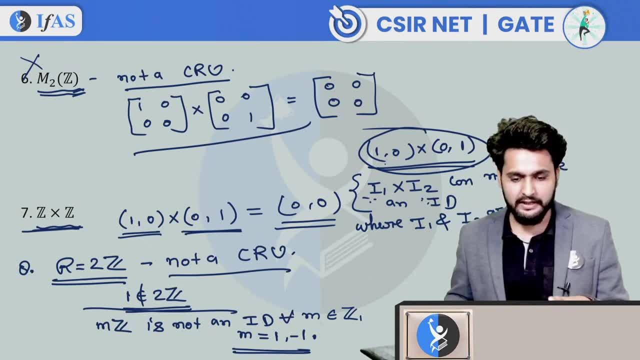 kabhi mz ke pas, kabhi bhi 1 nahi hoga, CRU nahi hoga to integral domain, kabhi bhi nahi hoga. umeed hai aapko clear hai, to integral domain vane ke liye 2 cheze. 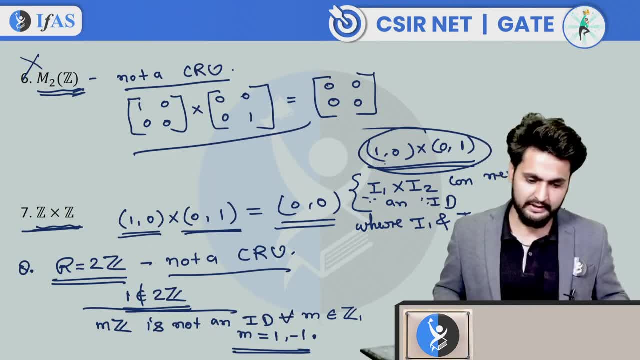 zaroori hai CRU hona aur ek bhi zero division nahi hona. agar aisa hota hai to integral domain, bach jayega. this is all about integral domain. kuch ek aur ins dekhte nahi apke integral domain. 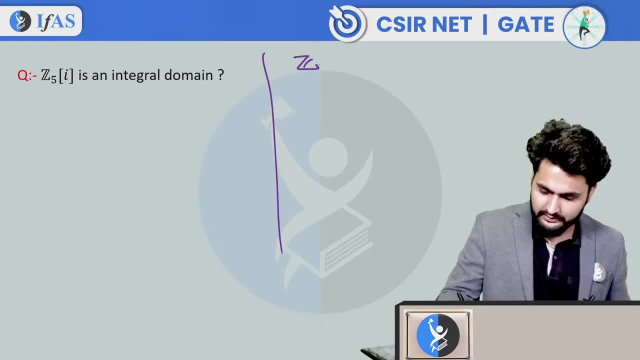 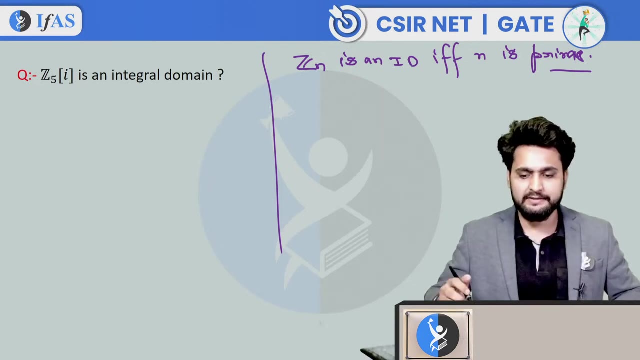 ki baat karte. jaise, abhi, maine aapko kya bataya tha? ki zn. zn is an integral domain if, and only if n is prime. but kya zn i ke liye sufficient condition nahi, agar aap bunti. 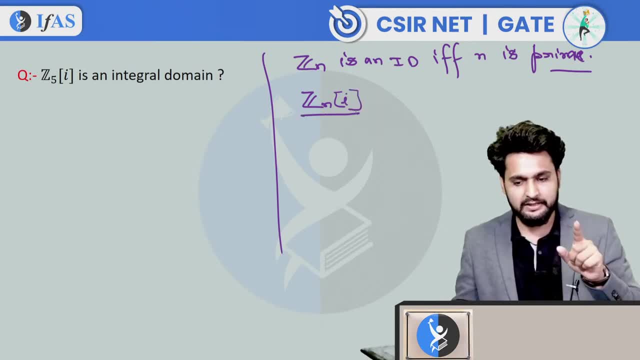 ho ki zn. i is an integral domain if, and only if, n is prime to wo galat hoga jese yahi pe dekho. z5i is not an integral domain. is an integral domain maine pucha apko and this is not. 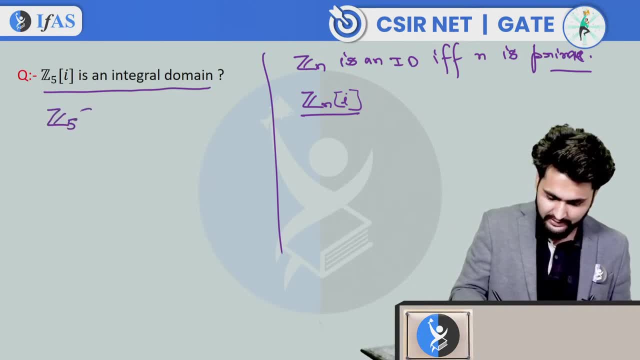 an integral domain, z, and i correct right. yeah, right, i got it. z5i is not an integral domain. ye integral domain nahi hai. ok, kyo kyun is ke paas zero division. mil jayenge kaun se zero division dekhi ek. 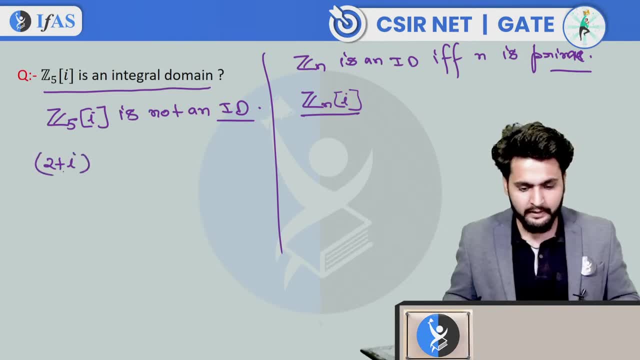 element mai leta hu. let's say 2 plus i. maine dekhi, aap 2 plus i z5i ka member hai. z5i ka koi bhi member kaisa hoga z5i. let me write here: z5i. 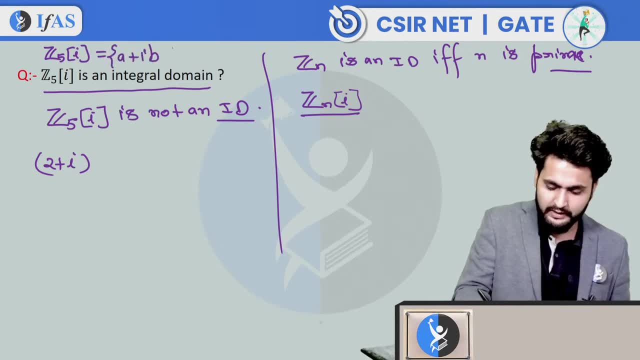 is defined as a plus i b, where a comma b belongs to z5. ok, remember, hai agar me 2 plus i into 2 plus i, 2 bar karta hu. let's say 2 plus i into 2 plus 2, non zero element. 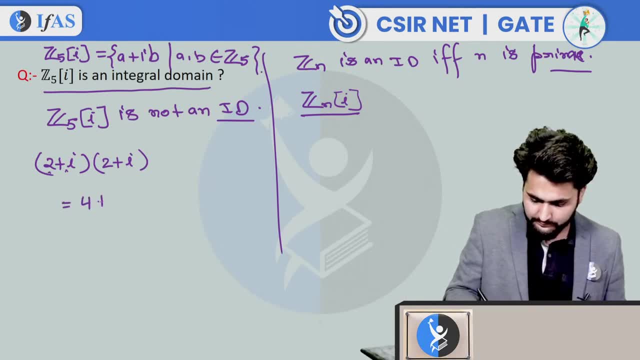 hai in ka product. dekho zera, kya milega: 2 to the 4 plus 2 i, and then 2 i, again plus 2 i and minus 1. i think issse nahi banega to kuch aur leta. 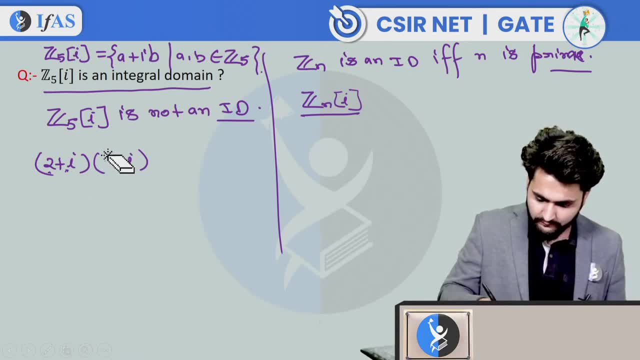 hu me. let's say isko kya karta hu me. 4 plus. i leta hu ek element dekta isle banega. 2, 4, 8, 4 to the 8 and plus, ktna ho jayega plus. 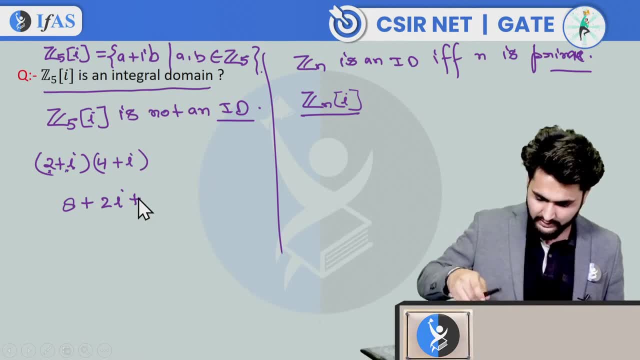 2 i and plus ka 4 i. issse bhi nahi banega. 4 i milega hume, and then plus ka 2 i, ek second dusa element dekta koi bata nahi, jayega koi zero. 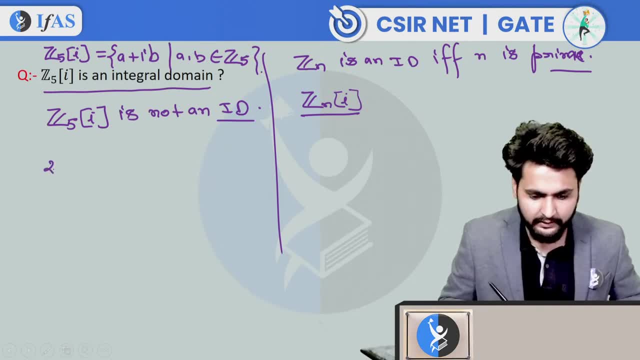 division. hum kya bana sakte, iska agar me. let's say 2 plus i zp is an integral domain. play a prime, b is prime correct, but z and i ke liye hum nahi bol sakte, iska zero division banane. 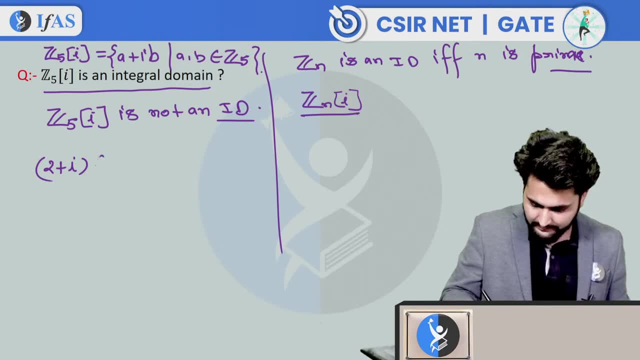 ki koses kar hai ek to 2 plus. i maini liya iske sa dusra element. mai kya lu ta ki dono ka product kare par zero a jaye aur z5. i ka hi member ho. na chayai to. 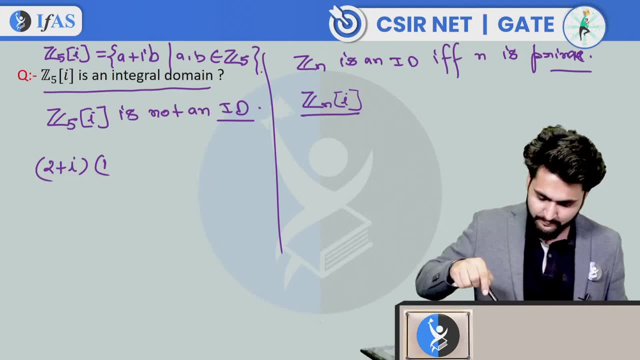 main, let's say, agar me leta ho. let's say, for example: if i consider, let's say 2, 2's of 4 and plus, let me say zero division, batana chayai, iska mujhe to philal nahi dekha. 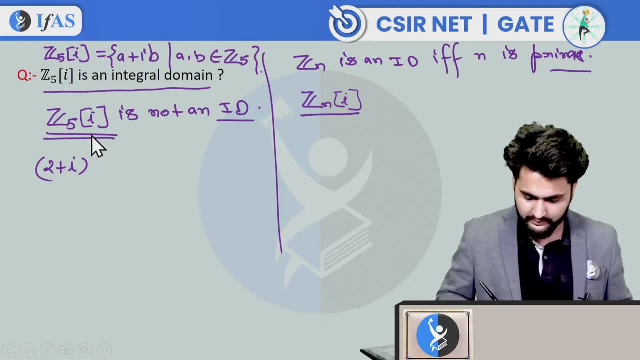 hai to plus i and 2, but we can have zero division, right? let's say we can have zero divisions in z5i. So what can be done? 2 minus? i See 2 minus i is not actually an element. Now it is right, You can say 2 plus 3i. Let me consider this. 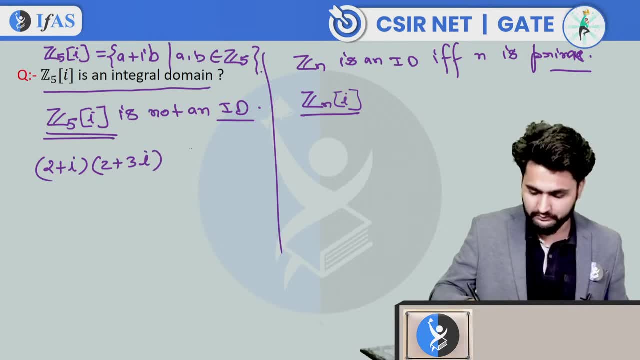 is 2 plus i into 2 plus 3i. If I take, then what will happen? Let's see So: 2 to the fourth and 2, 3, just 6i right, Plus 2i, plus 2i and minus 6.. I think this will not. 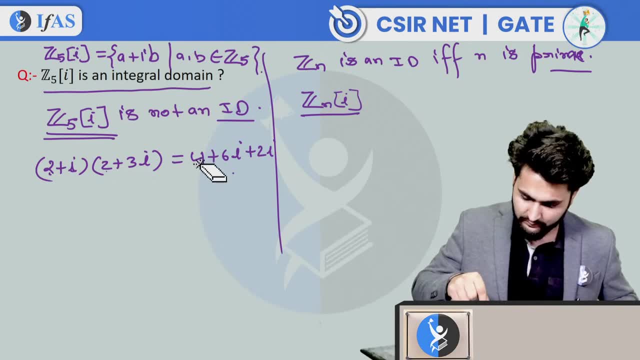 work. We have modulo 5, so this does not work, it seems. Can you consider something else? 2 plus 3i will not work, 2 plus i and 2 minus i, 2 to the fourth plus 1.. Let me check it. 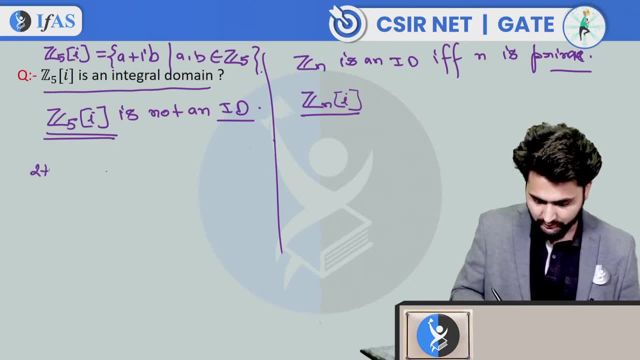 once They are zero divisions, 2 plus i into 2 plus 3i. If I take, then what will we get? 2 to the fourth and 2, 3, just 6i Later. I will take it as modulo, So let's assume. 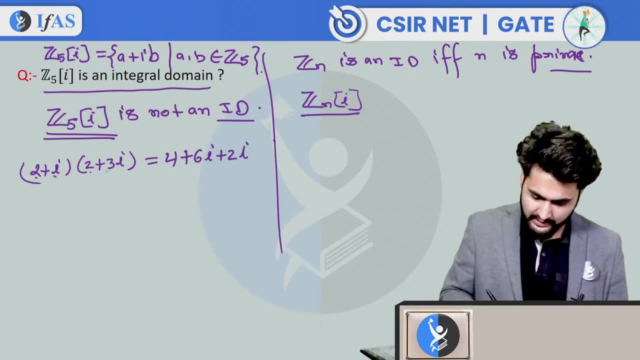 that it is 6i and plus 2i and minus 3.. Right, This will not work. Can we take something else: 2 plus 4i? I think? right, It will work. Let's see. If we take 2 plus 4i, it will work If. 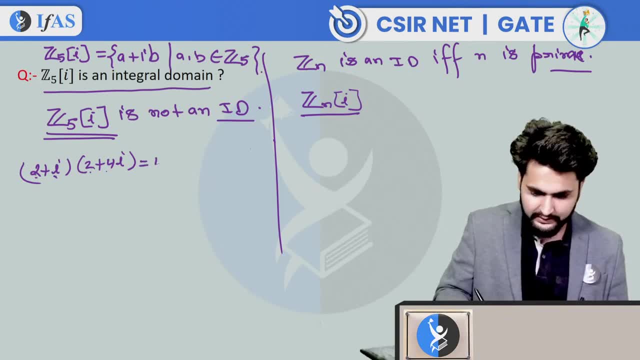 I consider this. then what will happen? 2 to the fourth. I think this should work right. How did you take? Yes, that's what China said, right? 2 minus i: we cannot take. This is what I said. Z5 will not actually be a member, right? If you take minus, then minus 1 means. 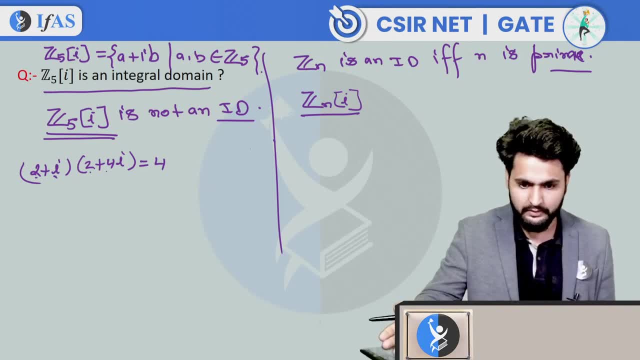 minus 1.. 1 means 1's inverse in Z5, which is 4.. So we can take 4,, right? So this will be 2 to the fourth plus 2 to the fourth, 8i, 8i. this will work And i into: 2 is plus 2i And this. 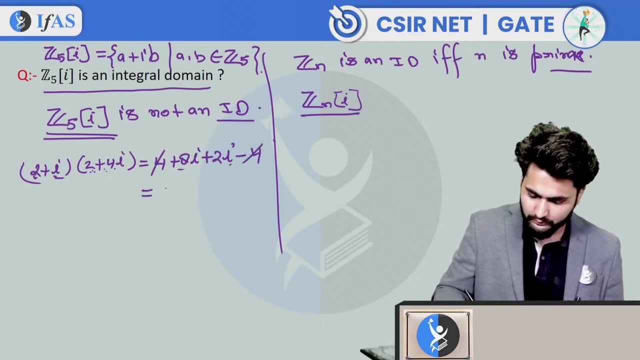 will be minus 4.. So this will be cancelled out. 2 plus 8 plus 2i is 10i And 10, what will we do? We have to take modulo. Where are we In Z5.. So we will have to take modulo. 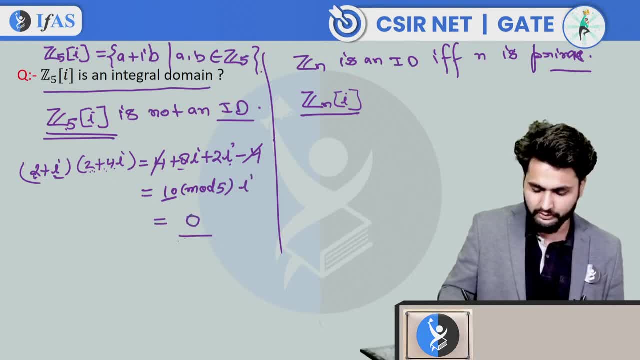 5 also, and then i So this is equal to zero. We have these two non-zero elements of Z5.. What will happen when we product them? What will happen when we product them? What will happen if Z5 becomes 0?? Ezome becomes zero. It means this is not an integral, So what? 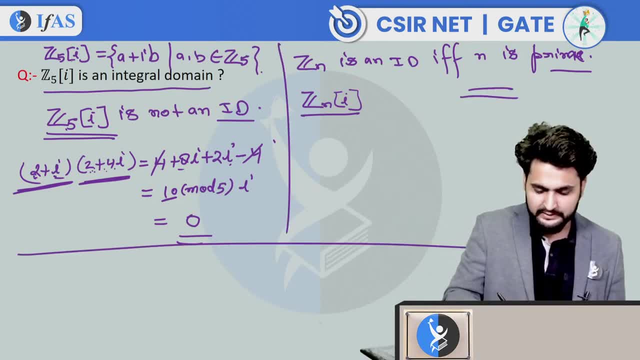 conditions can be for znak n for an integral domain like zna for it. Although there are some conditions for znai, There is absolutely one and that is the condition which I told you earlier: ZNI is an integral domain if, and only if, n is prime And n is congruent. 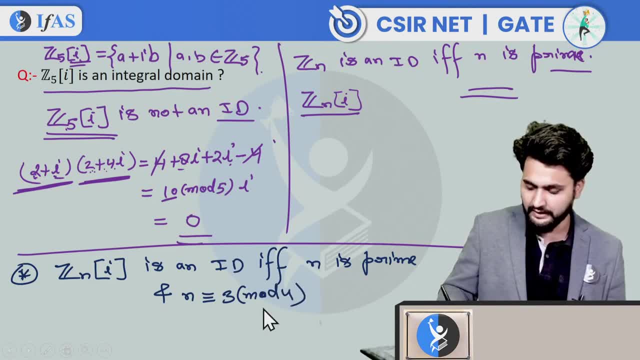 to 3 modulo 4.. So being only prime is not enough anymore. After calculating z, the utmost, the norm of the integral domain will be zours, Soромins, similar to the Sum of n equals 1 and n is prime as well. That is, the professions were also toình- uniform v's and as this figure 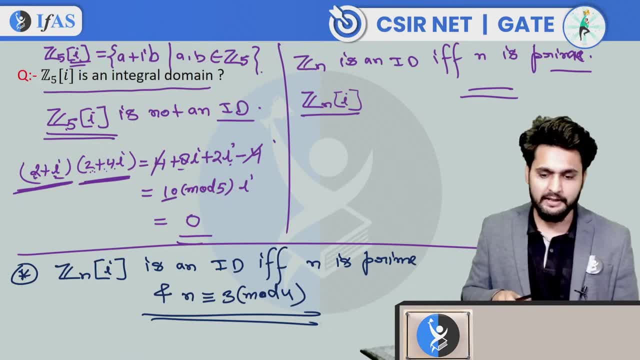 Now you will need two conditions: n should be prime and n should be congruent to 3 modulo 4.. If I divide n from 4, then remainder 3 should come. Now I am not verifying this, but if you are interested, then this can be verified. 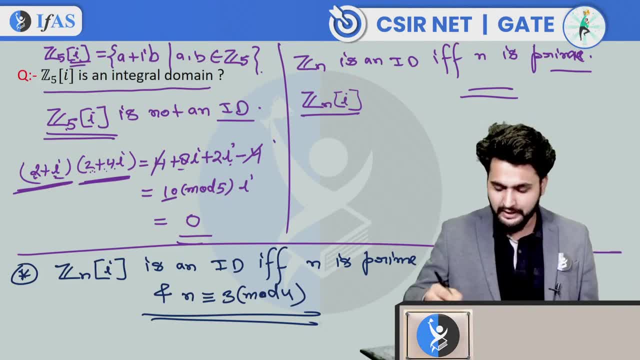 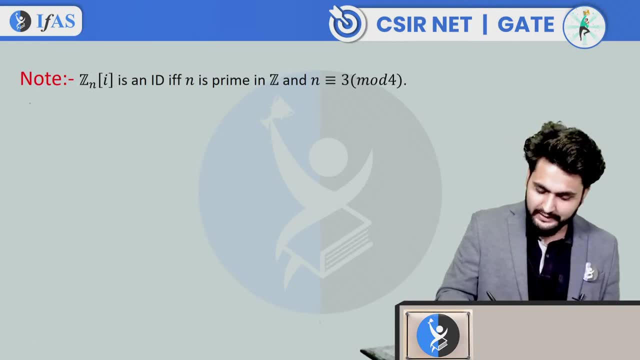 Zn i is an integral domain if, and only if, n is prime and n is congruent to 3 modulo 4.. I hope you all will be clear. Like there is a note which I have just told you. actually it is written there: 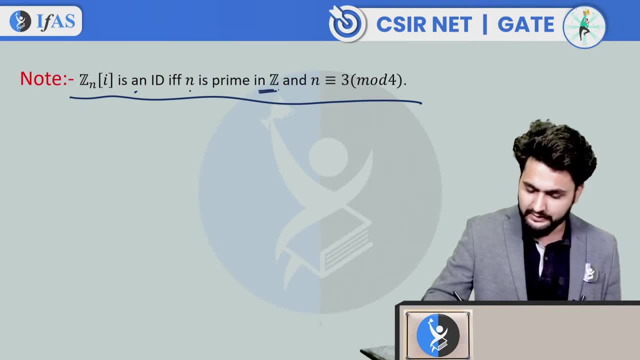 Zn i is an integral domain if, and only if, n is prime and prime in z and n is congruent to 3 modulo 4.. So z should be prime in z, because you can define prime anywhere. That is why it is written that n should be prime in z and n is congruent to 3 modulo 4.. 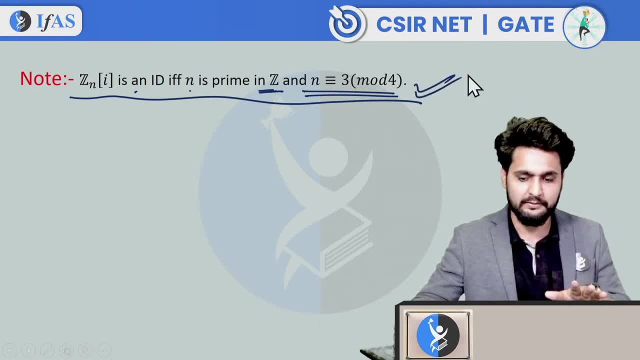 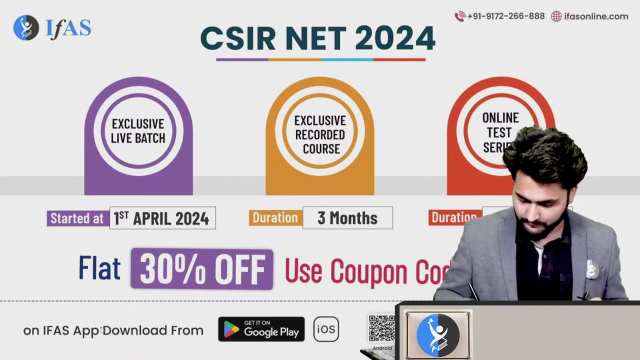 So if both are conditions, then zn i will be an integral domain. Otherwise, it is not necessary to have an integral domain only if it is prime in z. Now let's move ahead. Before moving ahead, let me tell you all: if you want to join us, join IFES with CSI N. 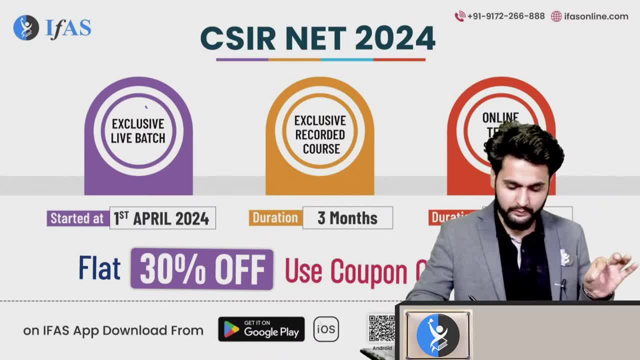 if you are preparing for a date. if you want to join us, then you can join us in three ways. You can enroll in live batches. If a new batch starts in one batch, you can join it with 30% off. You have to use the promo code IFES30.. 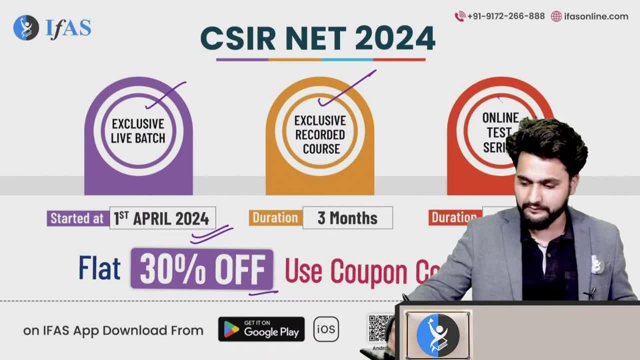 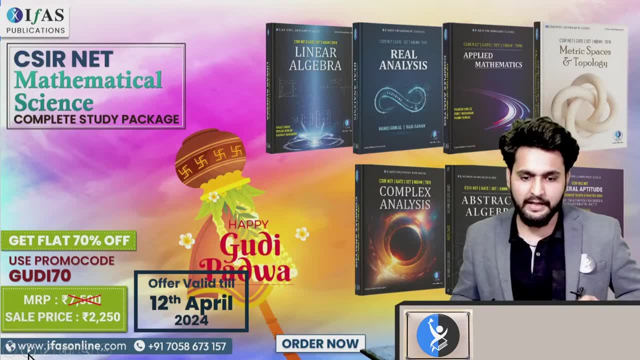 And a recorded course is also available. You can buy a recorded course or you can buy an online test series Along with that. if you want content, if you want books, then a complete package is available for you with 30% off. 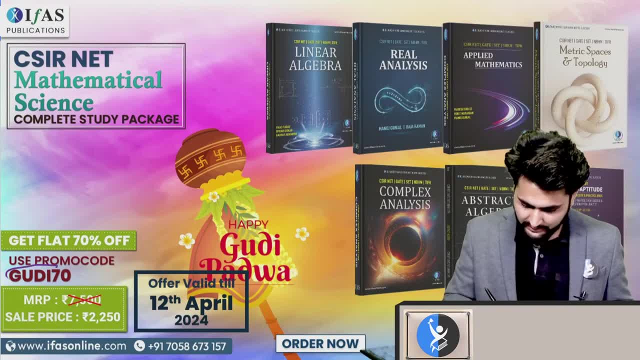 There is an offer of Gudi Padwa. So what you have to do with the promo code Gudi70.. If you use Gudi70, then with 70% off you can buy a complete package of a total of seven books. 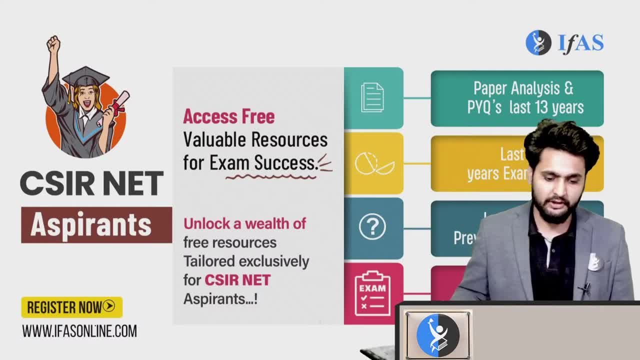 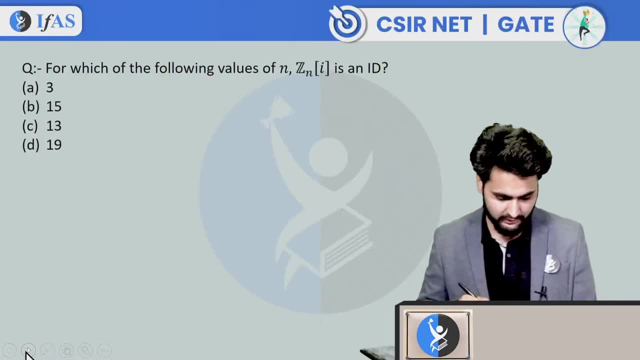 And you can visit our website, ifsonlinecom, where all the information related to the exam is absolutely available for free. You can access it and prepare in a better way. Okay, the next question is: tell me what can be the answer to this. 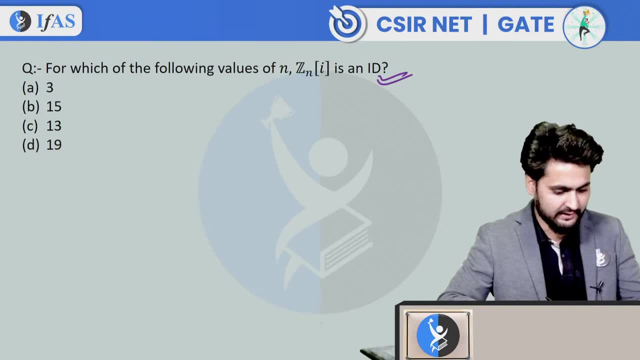 If you understand the last point, I told you what will be the answer to this. What do you think And which of the following values Of N, Z and I is an integral domain? Answer it quickly. By the way, I have asked you this question many times before. 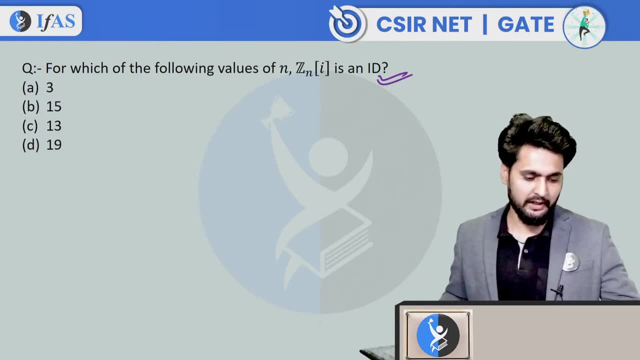 What will be the answer? When will Z and I be an integral domain? What value do you consider for N? What do you think For which of the following values of N, Z and I is an integral domain? When will Z and I be an integral domain? 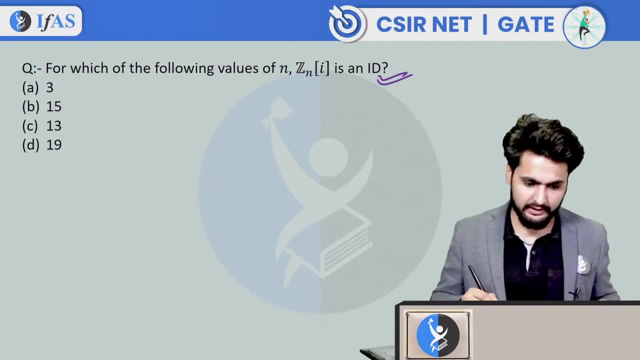 You are thinking of D option right. Check all the options. then you tell me: okay, You are thinking of C. Okay, Frank, you think B and D are correct. Everyone is thinking differently. Have you read carefully what I told you? 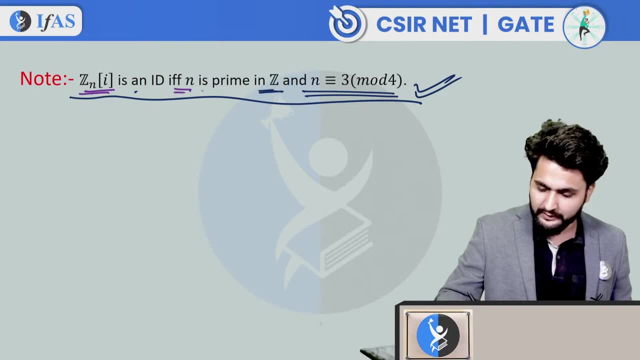 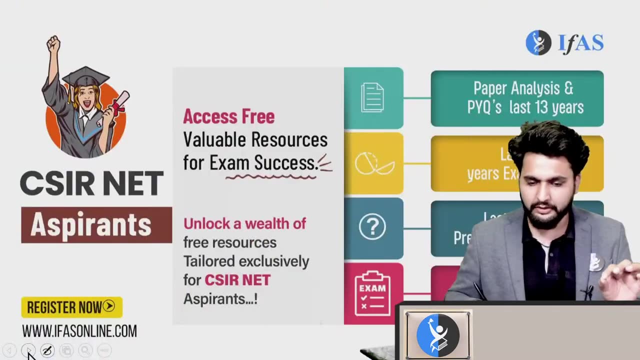 Z and I is an integral domain if, and only if, it is prime and congruent to 3 modulo 4.. Both things should be there. N should be prime. If you divide it by 4, then remainder 3 should be there. 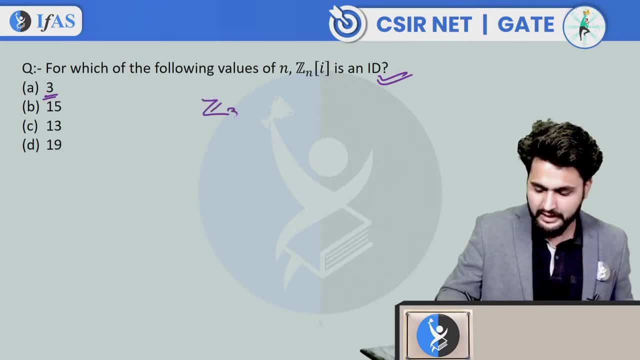 So is there any problem in 3?? Is there any problem in 3?? If I take Z3i, then what is the issue with this? Is there any issue? 3 is a prime number. 3 is a prime number. 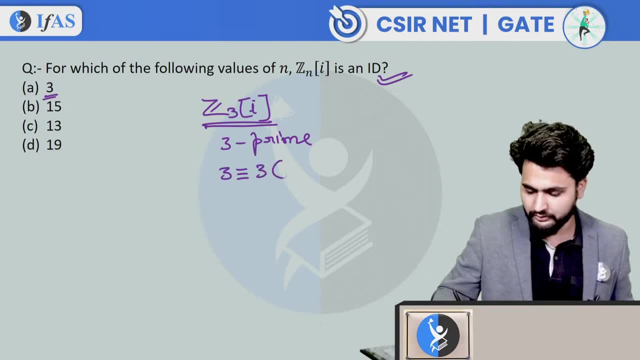 If you divide 3, this is congruent to 3 modulo 4.. If you divide it by 4, then remainder 3 will be there. What is the issue in 3?? Prem, Premkash, Shanta, Azit and everyone, what do you think? 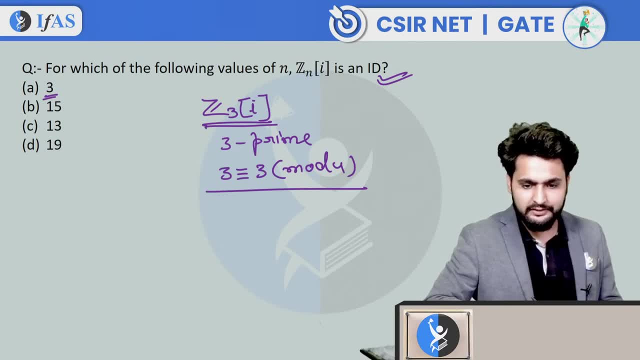 Can't there be an integral domain for 3?? So Z3i will also be an integral domain. What is the problem with 3?? How can it be 15 if you are answering B and D? This is not a prime number. 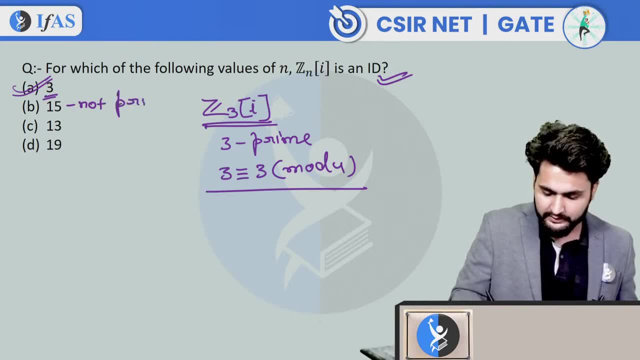 The first thing is that it should be prime, not prime. This is not prime. If it is not prime, then how can it be? Remainder 3 is a good thing, But first of all, it should be prime. If it is not prime, then how can it be? 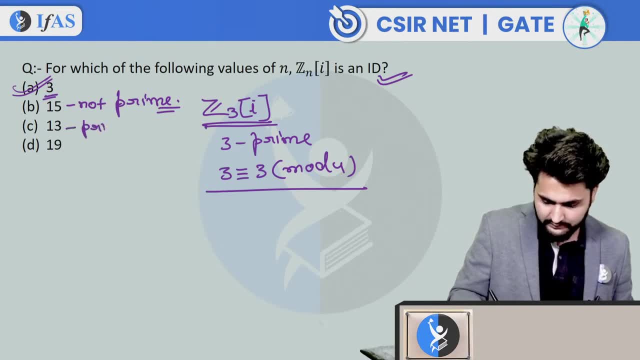 13 is a prime number. This is prime. 13 is a prime number. But the problem with 13 is 13 is not congruent to 3 modulo 4.. If I divide 13 by 4,, 4, 3 is 12 and 1 is 13.. 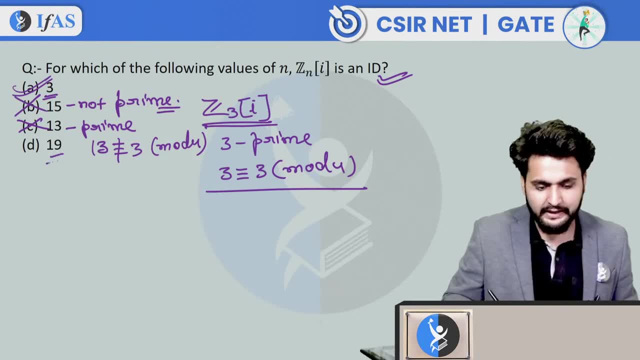 1 remainder will be there. So this is not. this can also not be. We can also consider 19.. So both A and D should be there. Azit Chena Munasha. Both A and D should be there. 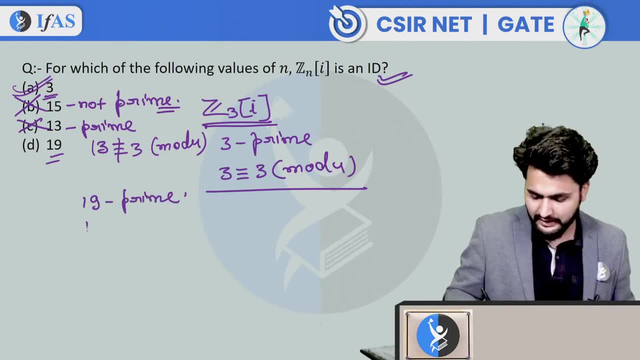 Because 19,. this is also prime And 19 is congruent to 3 modulo 4.. If you divide 4 by 4,, 4 is 16 and 3 is 19.. So both of these are your correct options. 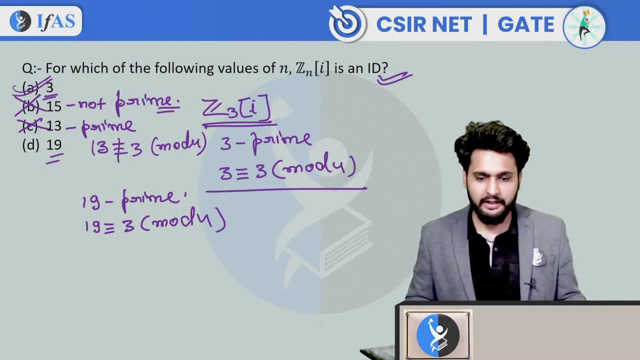 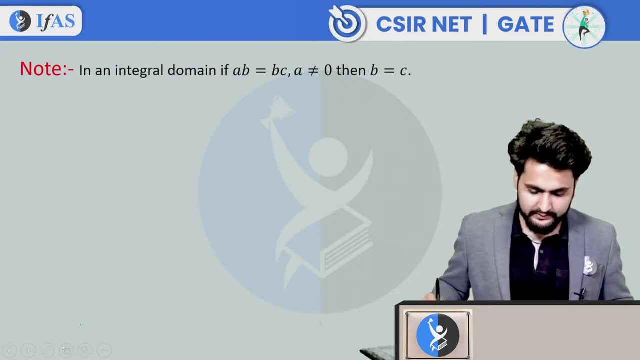 Is that clear? Yes, Fine, Priyanka. A and D are the correct options, So you don't have to do anything wrong. A and D are the correct options. Now let's move ahead. Next point is in an integral domain. 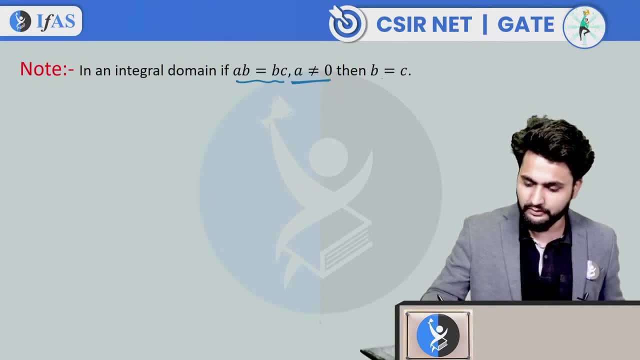 if AB is equals to BC, A0 equals to 0, then B is equals to C. Left cancellation law or cancellation law holds in an integral domain. If you have an integral domain and in some way A equals to AC, 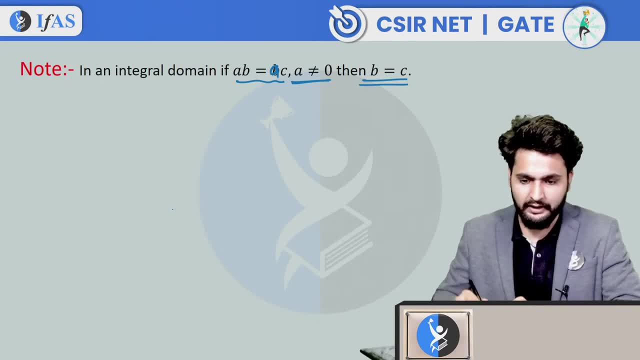 BC should not be there. AB is equals to. if AC is there, A0 equals to 0, then you can write B equals to C. If the cancellation law is not an integral domain, then it is not necessary that it is valid. 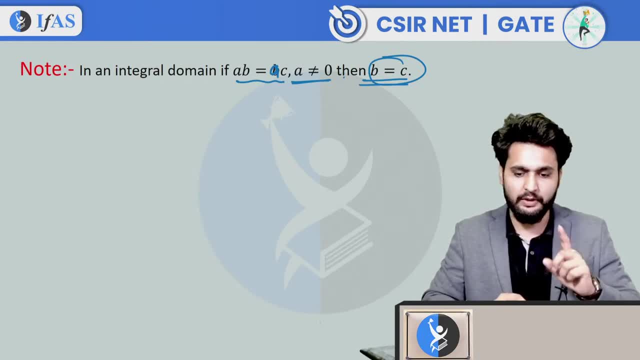 Okay, Cancellation law is valid only if you are in the integral domain, Otherwise your unit element should be there. See, If you take AB equals to AC, then minus AC equals to what I can keep 0.. If I take A commonly, 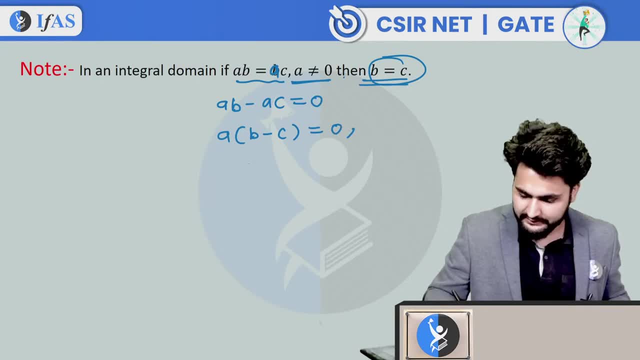 then what will I get? B minus C equals to 0. Now what do we know? Since A0 equals to 0, implies that it has to be 0. If you were not in the integral domain, then you could not have said. 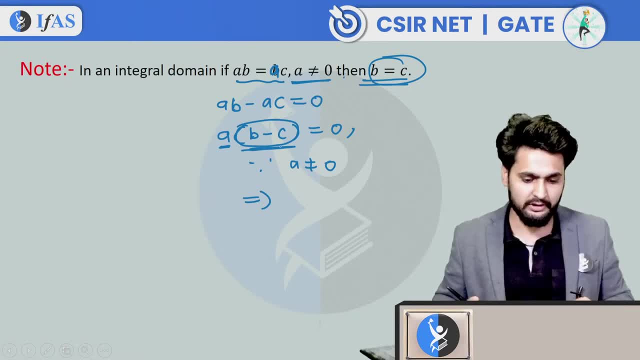 It is possible that this is also non-zero. This is also non-zero. Even then, the product is getting 0. Because we are in the integral domain. that is why we are able to apply this: B minus C equals to 0,. 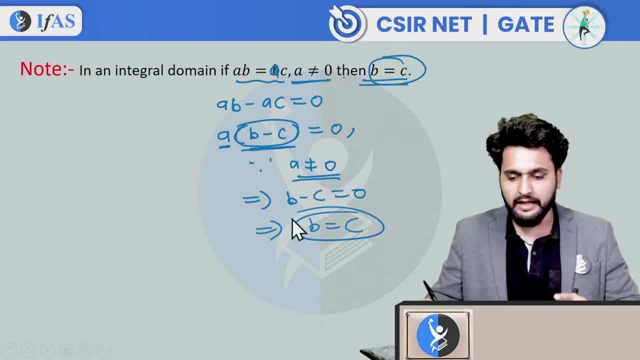 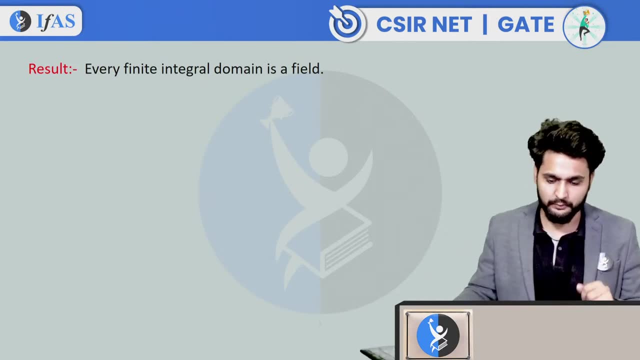 implies that B equals to C, So cancellation law holds in the integral domain. Okay, Fine, Now let's move ahead. If anyone is confused, you can ask me. Next result is: every finite integral domain is a field, As I was saying. 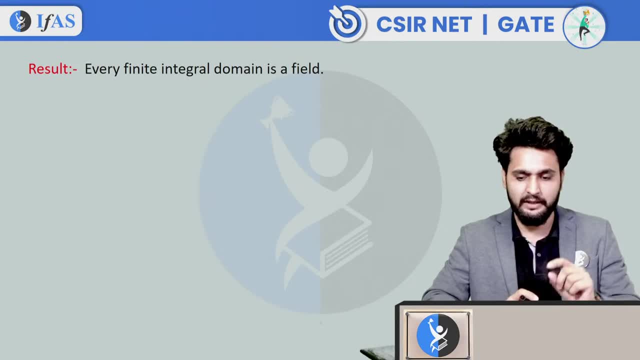 the last point I told you: in any finite CRU, every non-zero element, either unit element or zero divisor, can be proved very easily by using it. The finite integral domains are also fields. Let's see how. Let's assume: 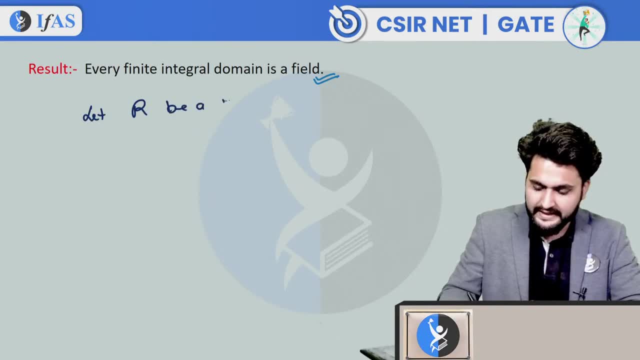 let R be a finite integral domain. Suppose it is a finite integral domain. If it is a finite integral domain, then CRU is done. What is field? Field should be commutative, ring with unity And every non-zero element should have a multiplicative inverse. 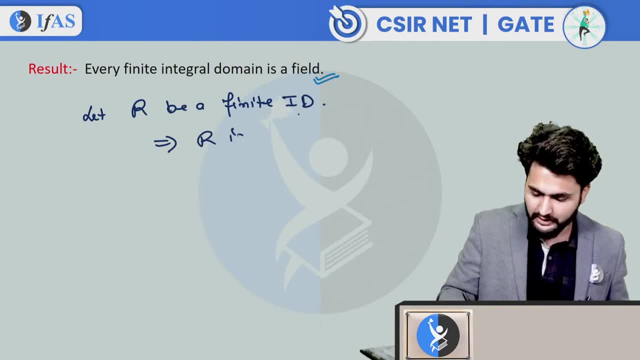 If it is an integral domain, then CRU is done, R is CRU. R is a CRU Commutative ring with unity. Now I want to show that every non-zero element will have an inverse. So I will take a non-zero element of this. 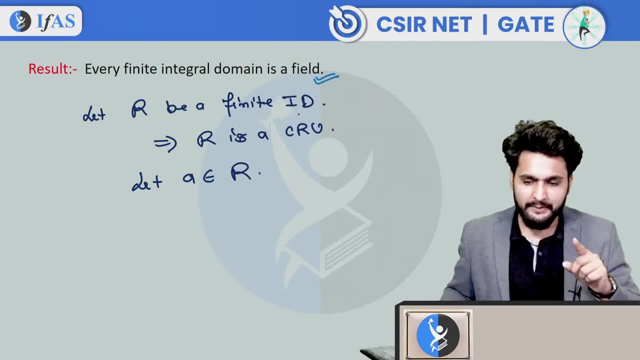 Let's say A belongs to R. I took A belongs to R Now, since R is finite, since R is finite, R is finite implies that finite implies that implies that what happens in finite CRU, Either it is a unit or a zero divisor. 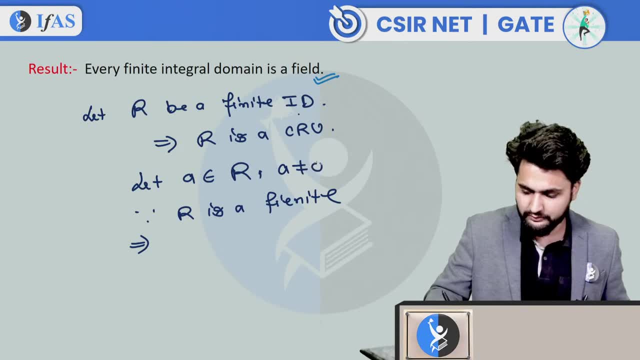 If you pick any non-zero element- let's say A belongs to R, A not equals to zero. Now I want to show that every non-zero element will be a unit element. So I took a non-zero element Because we are in finite CRU. 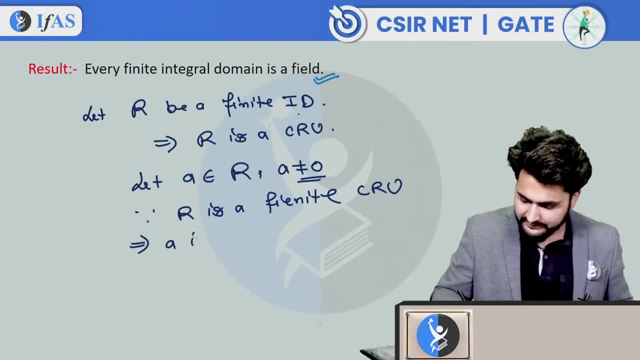 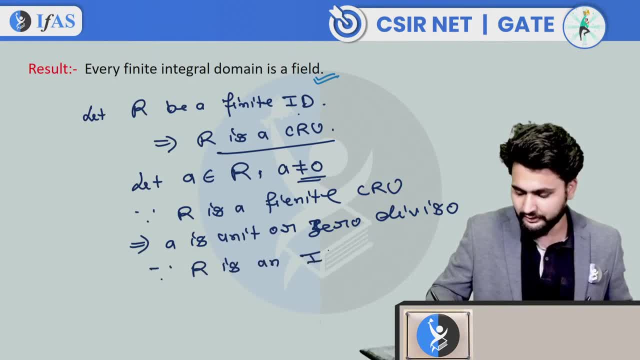 since R is an integral domain. R is an integral domain, so it does not have a zero divisor. What does this mean? It implies that A is unit. It has been proved. A is unit In finite CRU- any non-zero element. 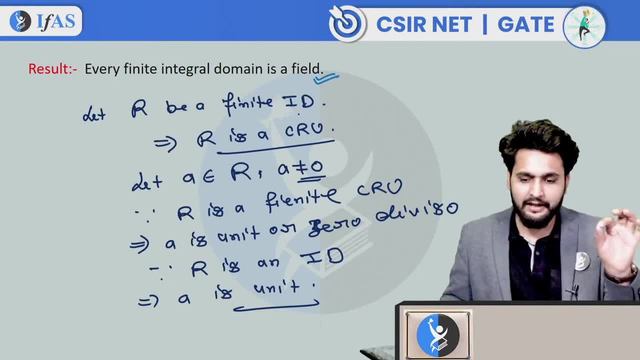 is either a unit or it is a zero divisor. Right, Because you are taking an integral domain along with the finite, So it cannot be a zero divisor. When it cannot be a zero divisor, then it means that every non-zero element. 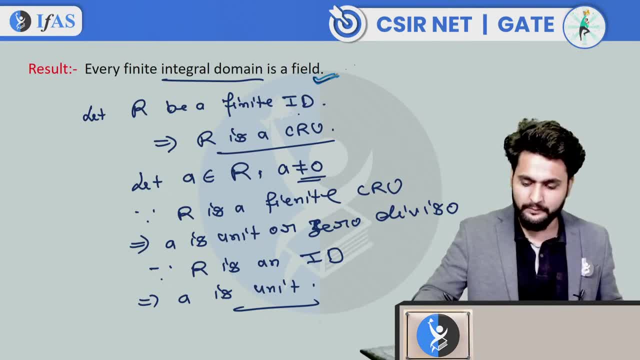 will have to be a unit element, And if this happens then it becomes a field. So any finite integral domain becomes a field, Right? So for z and i the condition: How is z and i? This is also a finite. 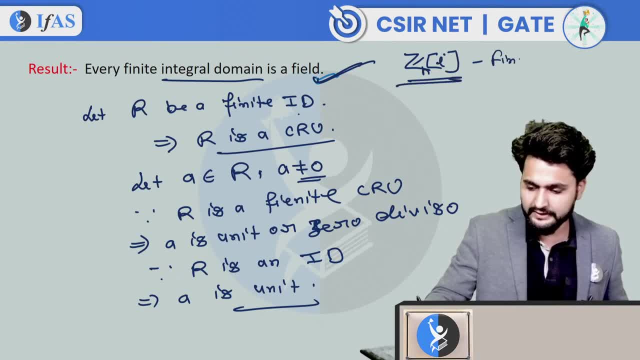 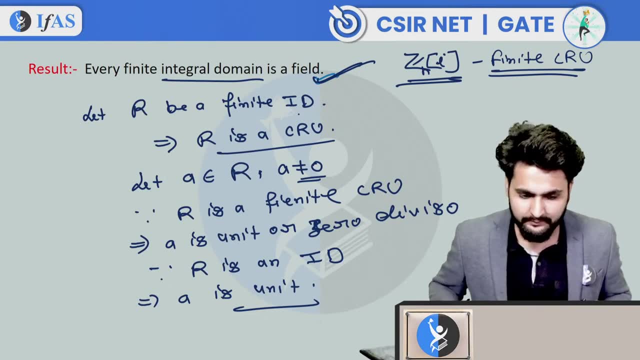 integral domain. This is also a finite CRU- Finite CRU- So the result for the integral domain was the same as it can be for a field. How can you write that z and i is a field if, and only if, n is a? 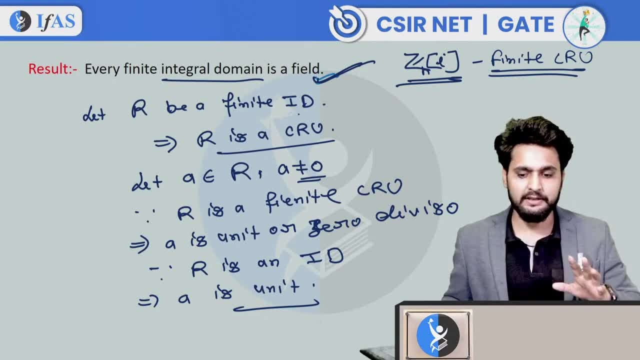 n is a prime, or n is a prime and n is congruent to 3 modulo 4?? So you can apply the same result for the field, because if it is an integral domain and finite, then it becomes a field too. Is that okay? 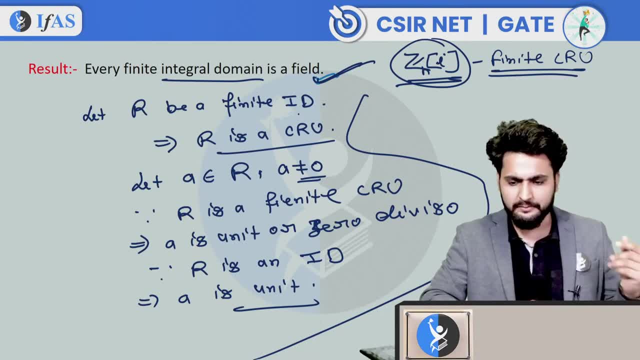 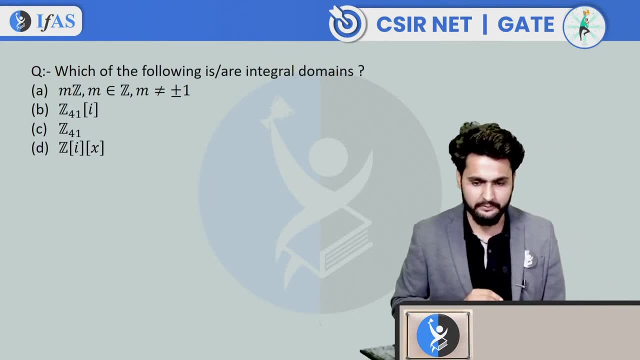 And the same result for z and i. z and i is a field if, and only if, n is a prime. You can say the same, because if z and i is an integral domain, then it becomes a field too. Fine, Look at this question. 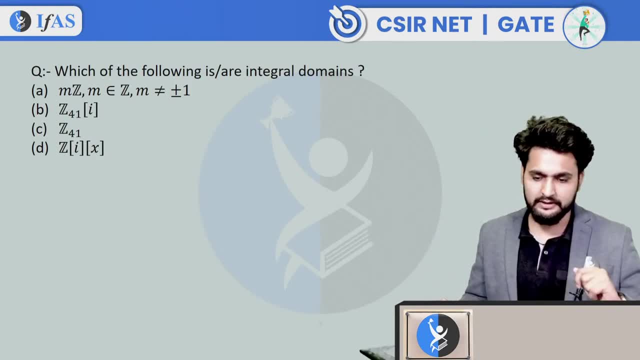 and answer it. This is our last question, Last question, and this is all about today's lecture. We will stop here for the day. In the next lecture, we will further discuss the topics for discussion. You know what the answer to this is. 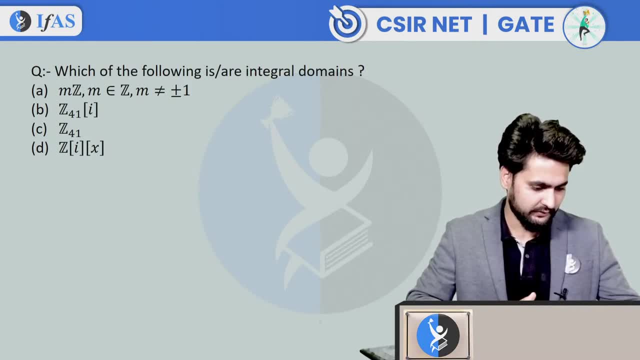 If you have listened to the lecture carefully, whatever I have told you, then answer it. What can it be? Next lecture means tomorrow. we will meet again at 5 pm. All of you have to join the lecture. Try to join it live. 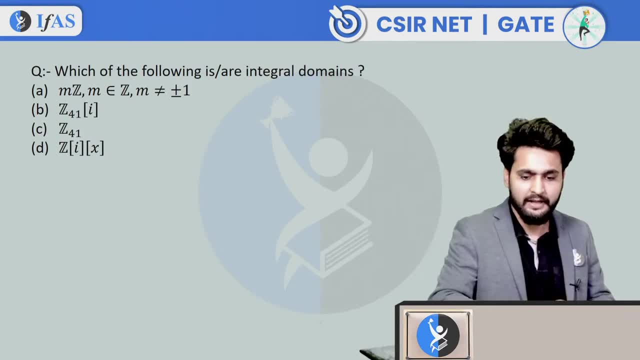 If you don't, then at least watch the recording. Later we will continue the video All the lectures in the last week. watch them once. In the next lecture we will meet at 5 pm tomorrow and talk about the principal ideal domain. 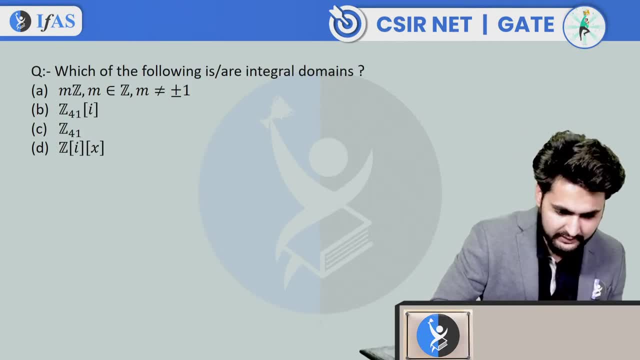 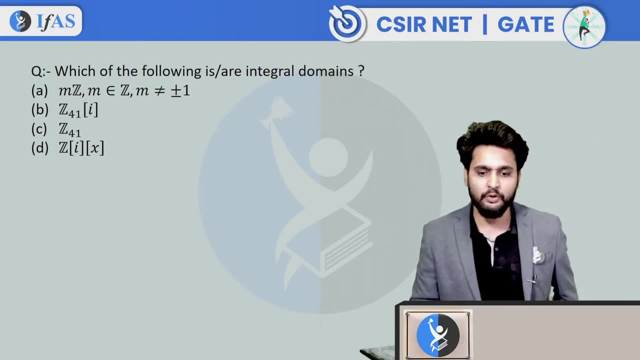 If you study a little by yourself, you will like it more. Ajit, do you think a and c will be correct? Shabna, do you think c is correct? The rest of the people will answer. What do you think is the correct option? 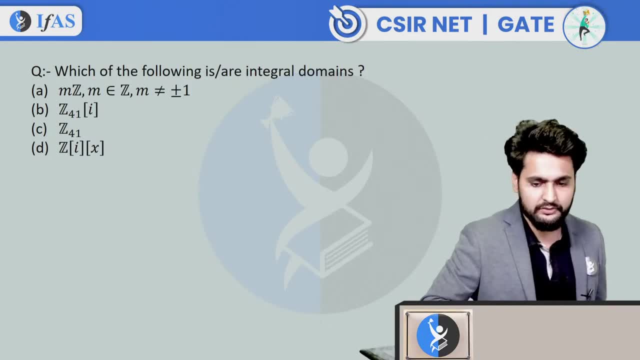 Which of these are the integral domains. mz m belongs to z. comma m is not equals to 1 comma minus 1.. If the integral domain is not equal to 1 minus 1, then it will not be 1.. 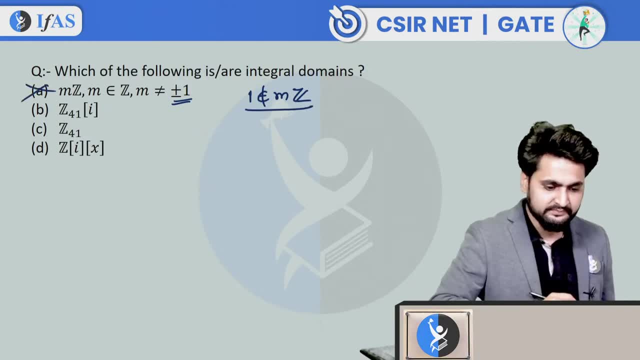 1 not belongs to mz. So how can this be an integral domain? How? How do you think a is correct? How can a be Shabna? you only think c is correct. Sayanta, you think c and d. 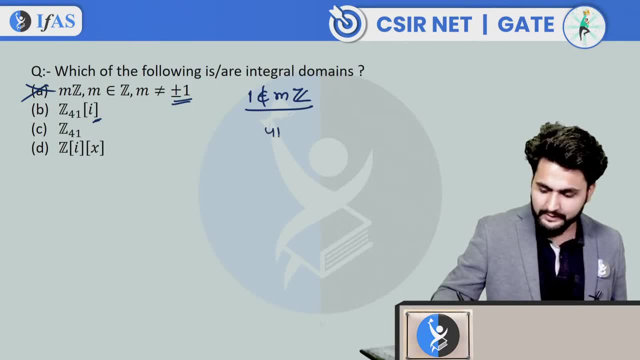 Okay, Fine, If I talk about b, z is 41.. 41 is a prime number. Very good, This is a prime number, Okay. Along with that, we need another condition: 41 should be congruent to 3 modulo 4.. 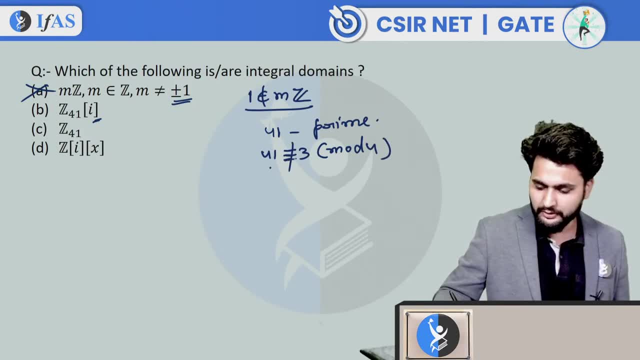 If you divide by 4, we will get 1.. So this is not congruent to 3 modulo 4.. So this is also not an integral domain. This is an integral domain. b will be your integral domain. What is the problem? 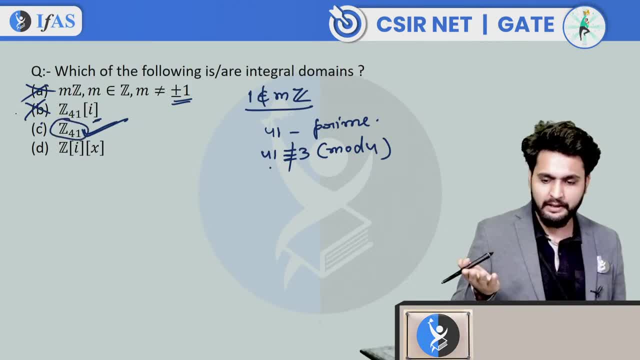 in that Right b is your integral domain. Why is it an integral domain? Because it is zn. zp is an integral domain. If only p is prime, then p is 41 prime. That is sufficient. So this is an integral domain. 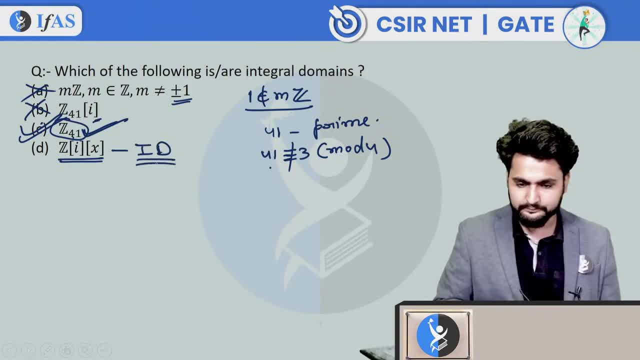 If I talk about zix, this is also an integral domain. So there is no problem in that. See how is zi. Do you know what is an integral domain? This is an integral domain. This is an integral domain, And. 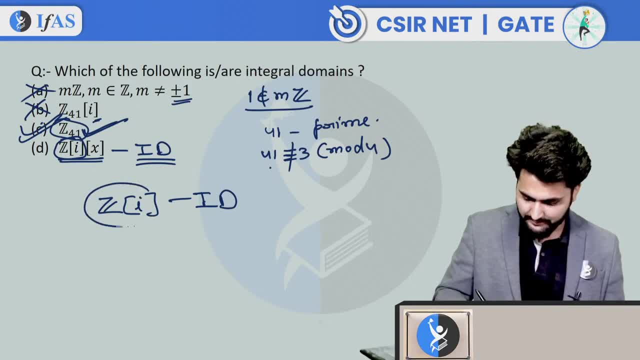 I just told you that if I make a polynomial ring from an integral domain, this is our ring r, And if I call it r, what will be? rx, zix, zix, Right, Because zi is your integral domain. 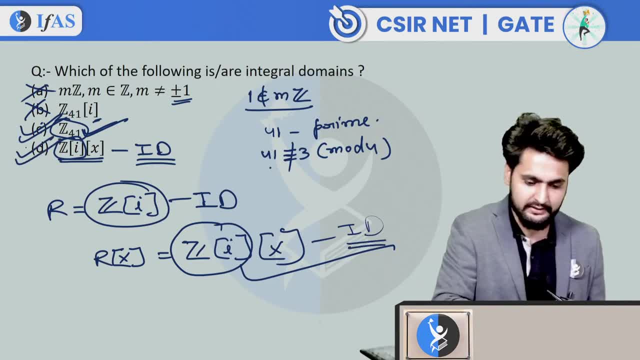 how is the polynomial ring zi and d is correct? Zina Pramka Pram. Is that clear to everyone, Is it fine? I hope you have understood, Manasha. ok, Now you are understanding that I have told you small mistakes. 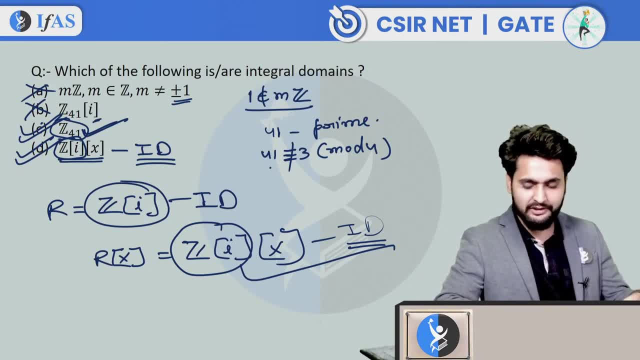 but you still have to pay attention to the lecture. you can see it again if you want. Try to understand that. at least these are very basic things. integral domain. If you see the questions of CSIR net, good questions are asked. 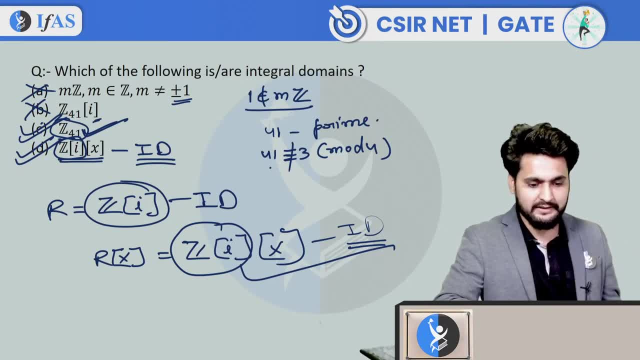 right. All things will be used in that, whatever is read till now. That's why we are reading basic things. You should not be wrong in this. ok, Thank you everyone for joining and we will meet in the next lecture. take care everyone.